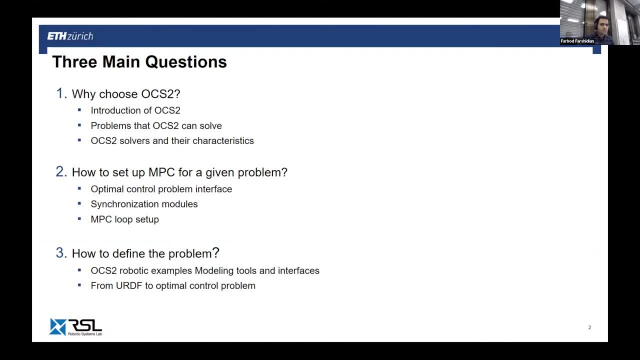 Then we will move on to see that. okay, if you have an MPC problem, it means that you have some system, you have its dynamics, costs and constraints, how you can set up an MPC loop, and on your real hardware or even in simulator. 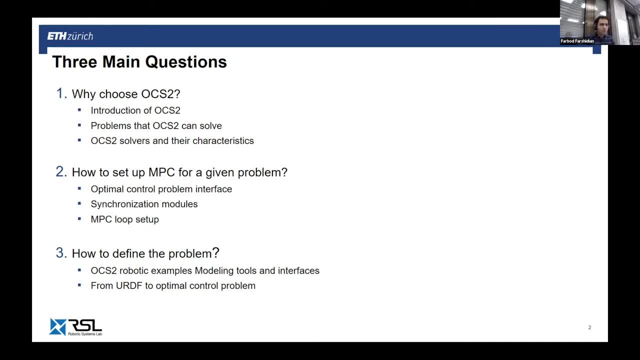 Then we move on to the last part. I'm going to talk about how OCS2 provides some tools to defining your optimal control problem Is that how it helps you to define your costs and constraints, And it covers some of the commonly used components of this optimal control problem. 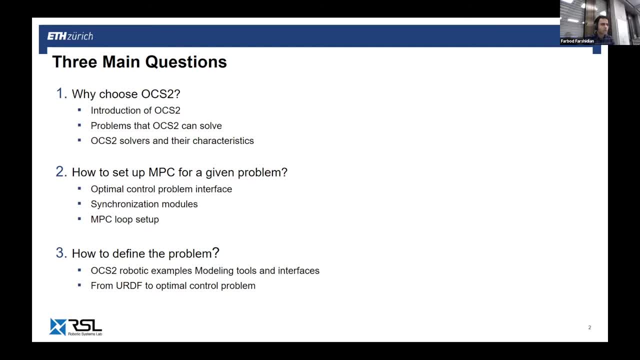 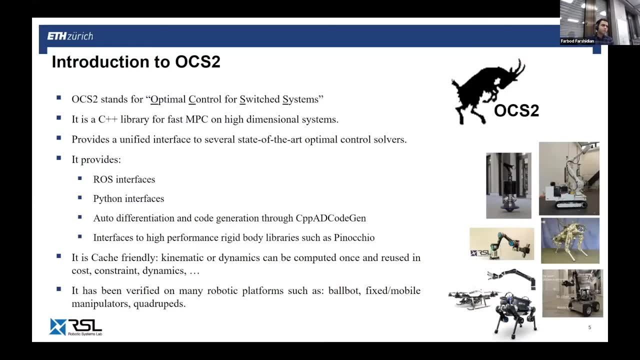 And I'm going to introduce this idea of the URDF2: optimal control. Okay, so we start with the first part. First of all, what is OCS2?? So OCS2 stands for optimal control for switch systems. It's a C++ library for efficient. 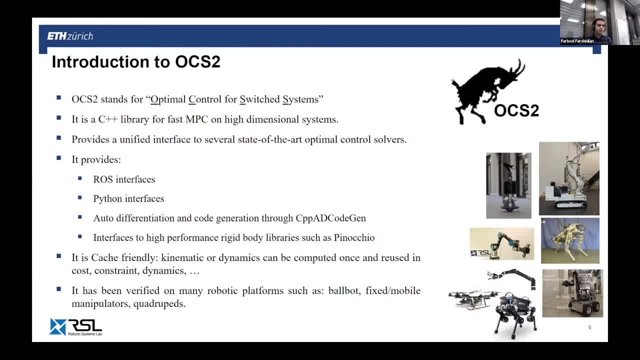 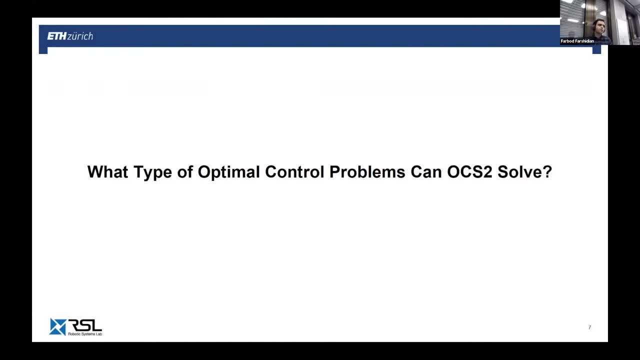 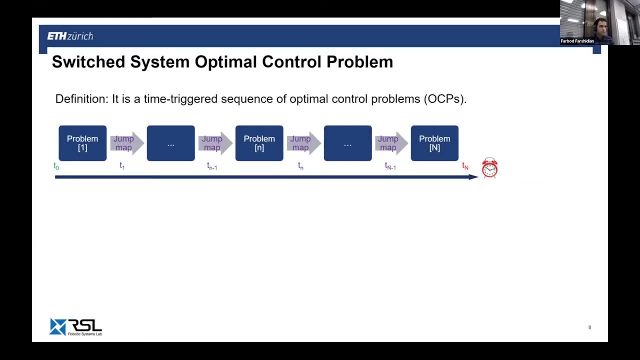 Okay, so now the next question is: what type of optimal control problems can OSC2 solve? So, as the name suggests, it solves the problem for switch system optimal control. So I'm gonna give it an official definition of that for switch system. 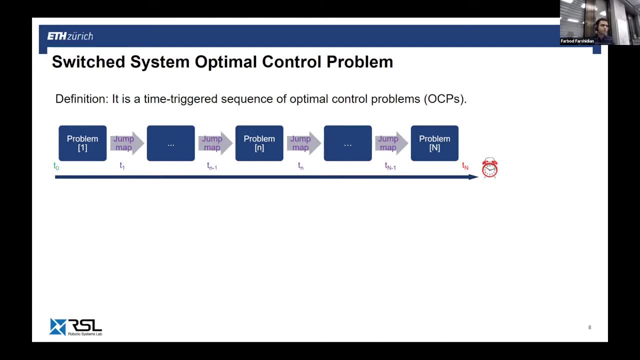 I will assume that it's a time-controlled sequence of optimal control problems. It means that you have problem number 1 to problem number N and at a given time you are going to change from one of these problems to the next one on some jump map. It means that the final state of one of these problems will go through this. 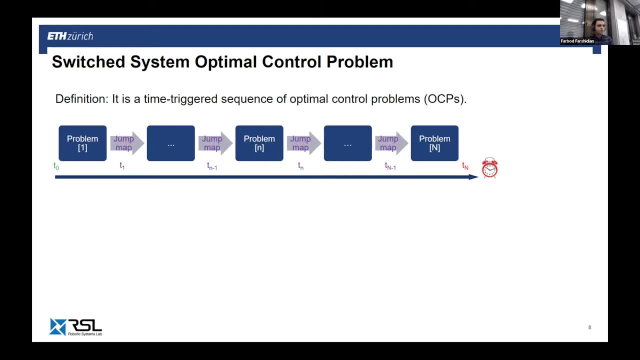 jump map and define the next, the initial state for the next problem. Times can be also optimized, but for sake of this discussion, let's imagine that the sequence and times are given. Now, what we will have here is for each of these problems, we can have this: our conventional thermal control problem. 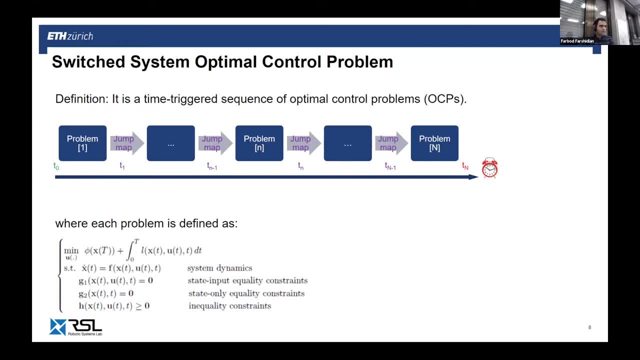 which consists of some some cost system dynamics, some state equality and equality constraints. I'd like to talk about a couple of terms here that you will see during this talk a lot. So, first of all, the first time we call it the initial time: nothing seeing, nothing strange. 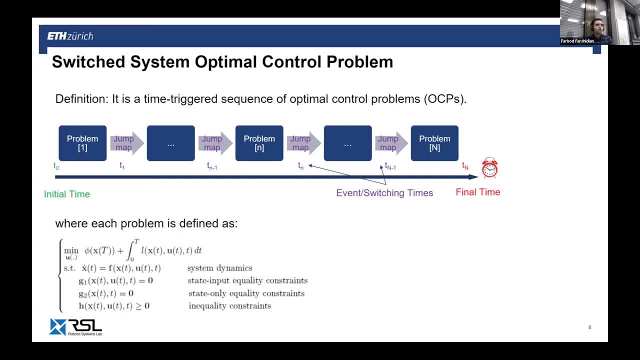 the final time called final and the intermediate ones are called as event or switching times and any time period between two switching time will be called as an intermediate times. So therefore in OSIS 3 you see terms like intermediate, cost and constraint. often we drop the term intermediate. it means that 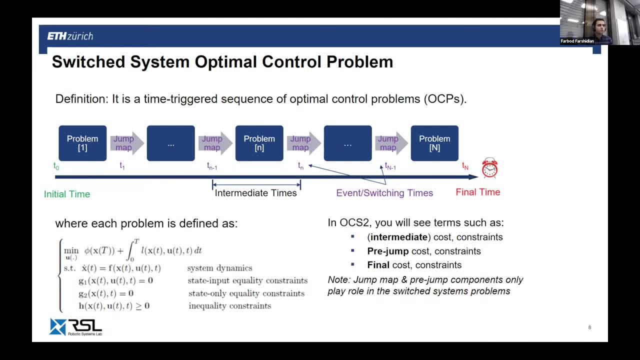 cost and constraints are effective during that. during between two to jump to switching times. we have pre-jump costs which are effective only at the switching times. but using the state before the jump map and also the final time, which, uh, which defines that? what would be the cost to go? 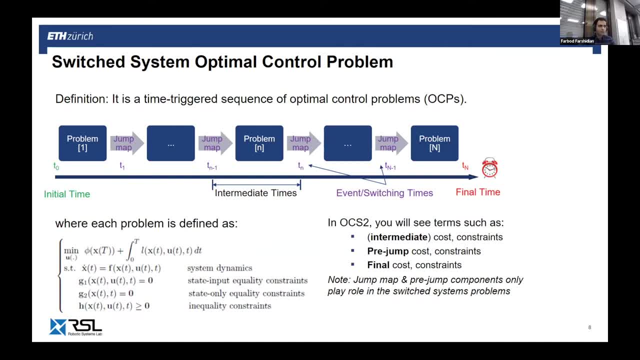 and some of the npc frameworks. they call this heuristic function. so you should note that this, the whole, this pre-jump cost and constraints or jump map stuff, just start to play a role when you're actually using a switch system problem. for a regular system you would just have intermediate. 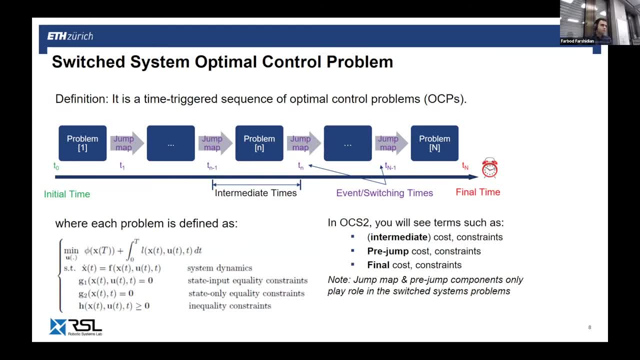 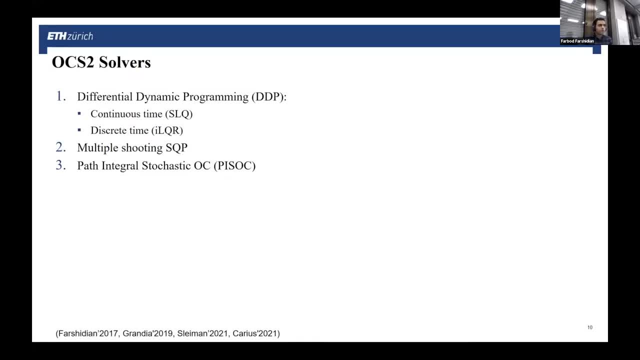 and final. okay, now next question: what solvers does osis2 use? uh. osis2 comes with three different solvers, um. so the first one is differential dynamic programming version, uh, which we heard about it in a previous talk. so it provides both continuous time domain version and discrete time, known as soq and iotr. it also provides a multiple shooting sqp. 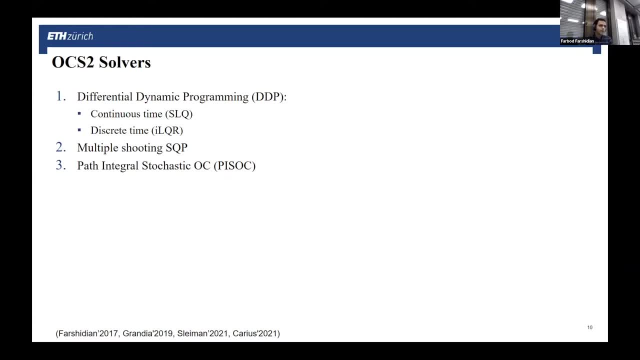 which is interfaces the backend with hbapm, and it also have a pass integral uh based optimal control solver, which is the- call it for sure, pisok. this is the only stochastic optimal control solver that we have in the toolbox. the other are deterministic uh. so of course we're not using the the original. 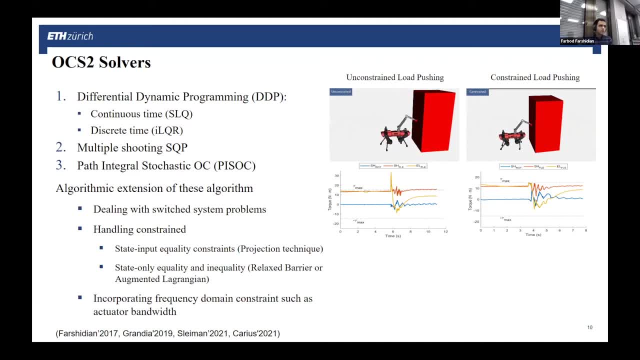 algorithm, most of uh. we did a lot of extensive attention to this uh. maybe the first and obvious one was we extended them to the work with the switch system and uh and, more importantly, we enabled them to handle constraints across the toolbox. we are always uh handling state input equality constraints through this projection. 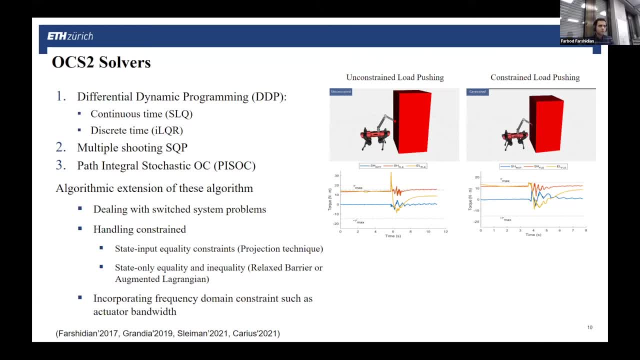 technique. that means that we use augmented lagrangians. uh, we define some lagrangians and then we resolve the lagrangian and define the problem in a lower dimension. it helps also for efficiency of the problem, for state only, quality and inequality constraints. either we use a relaxed barrier or augmented. 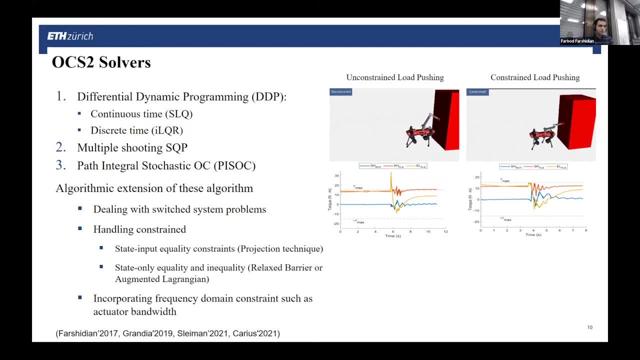 lagrangian technique. i'm not going to talk about the details but it's consistent across all the solvers uh, i mean, we tried it. this augmented lagrangian is the newest uh development of our group and we show here. we show some example of how it helps us to respect the uh, the joint limit. 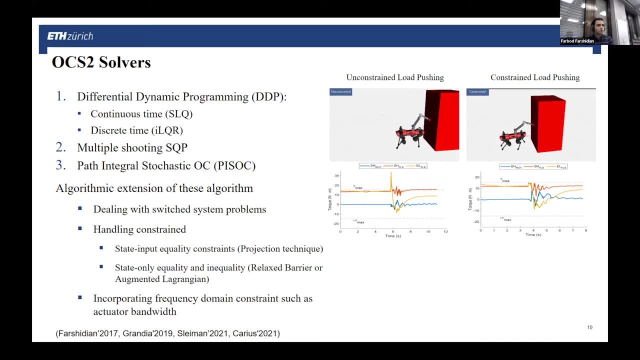 joint kinematics and uh torque constraints in in this uh box pushing task and the the final thing- this is the incorporating frequency domain constraints. um this. this is: this is a feature that you need to have if you're dealing with the real system and you want to implement your, your npc, on a hardware right. you just don't have temporary spatial. 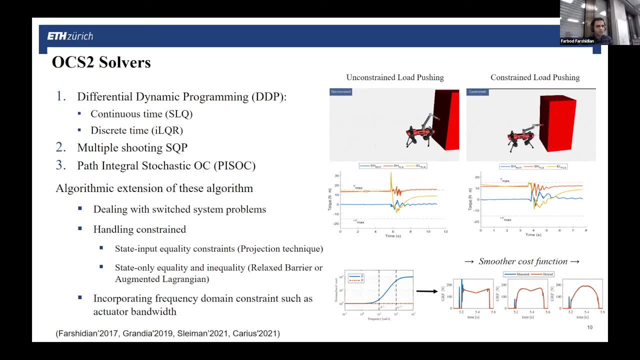 constraint like this pass constraint, you also have some bandwidth limitation of a heart of the actuators, so you want to have some tools to be able to put to to shape your- uh, shape your solution in the frequency domain means that i want to, for example, confine them in. 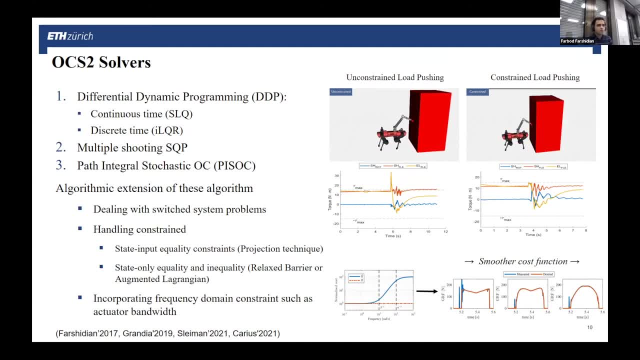 a lower frequency because they're actually cannot track high changes of the torque. so this can be done through this frequency domain approach and the nice thing is, once you define your original problem, you, by simple call off, create a frequency shape problem. you can create another problem which 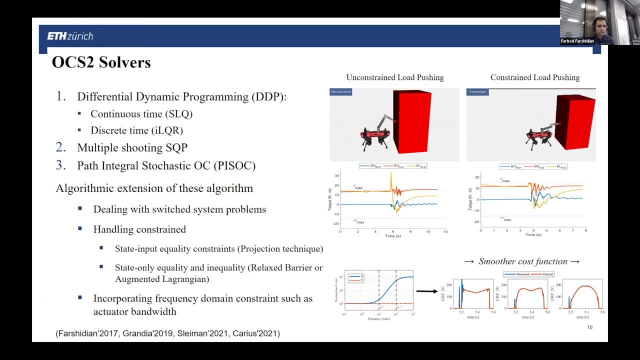 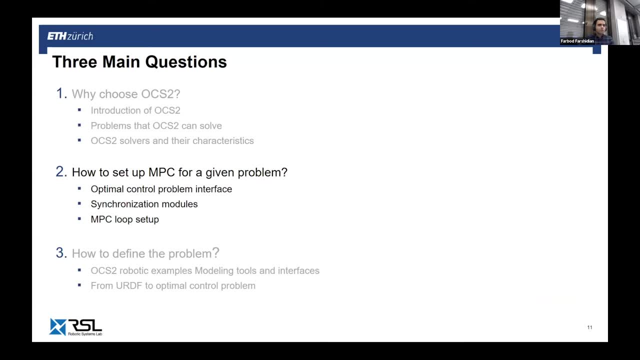 is, uh, having restructures or your dynamics cost and constraint in this area. okay now, i think with this we covered the main feature of this ocs2 and why what it has now. we will now move to next part, so how to set up an npc loop for your given problem in simulation and hardware. 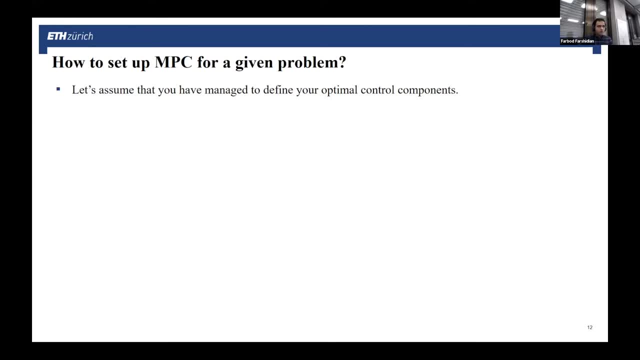 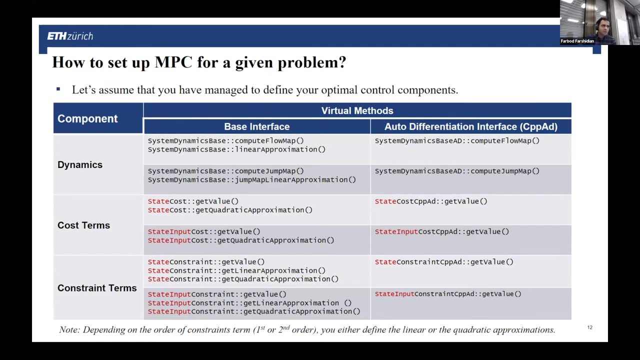 okay, uh, let's assume for now that somehow you drive your optimal control components. by that i mean that it's a c plus plus code, right, you need to derive from our base classes, our base interface classes and, uh, implement some of these virtual methods. so these components are dynamics, cost and constraint terms, right, as you see here. for 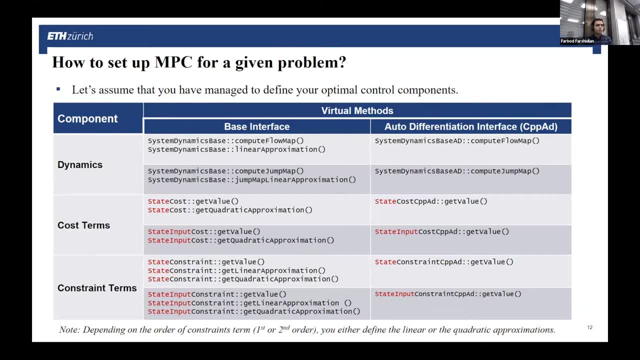 dynamics, you need to implement the compute flow map and its linearization and if you have a switch system, you also need to implement compute jump map and also it's linearization. but if you're having a regular, regular system, this you can ignore this part of course implementing linearization. 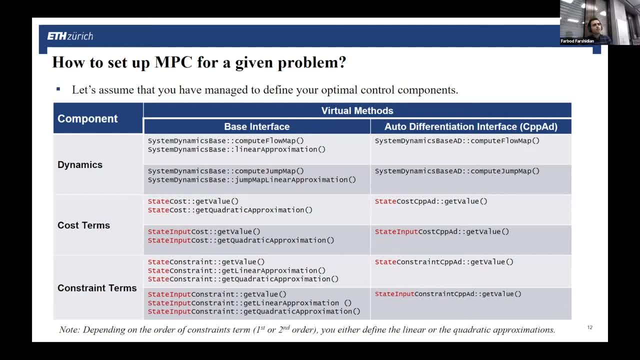 is by hand is not easy task, so that's why you also provide an automatic differentiation variant that you just need to implement. the value function evaluation- is it just a compute flow map or compute jump map? and its derivative are can are calculated through the solver internally. after that it comes cost terms. so in general cost can be just function of state or can be function. 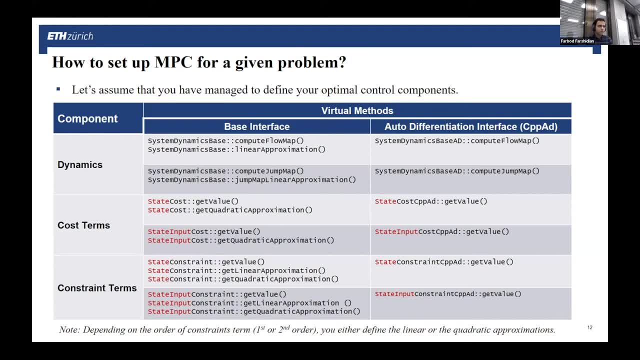 of state and input. you need to implement both the value and its quadratic approximation. again, you can rely on cpp, our auto differentiation, and just implement the function evaluation. and finally, it comes to the constraints. for constraints you need to do the value and linear approximation, or quadratic, depending on. 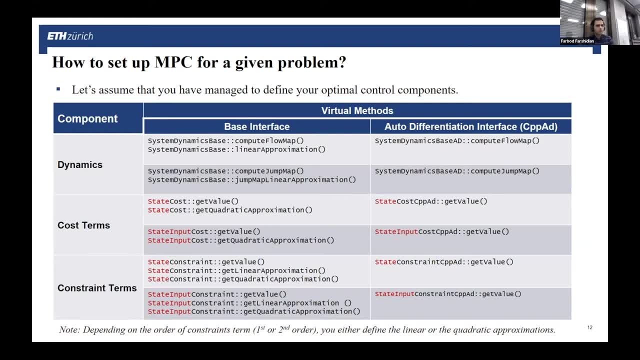 what order you want your constraint to be approximated. again, there's a cppad version now. let's for now think: assume that you implemented your dynamics, cost and constraint for your optimal control problem. now you have these components. now we will look into that- how we can set up an optimal control problem. so you need to take in general three steps: first, to set. 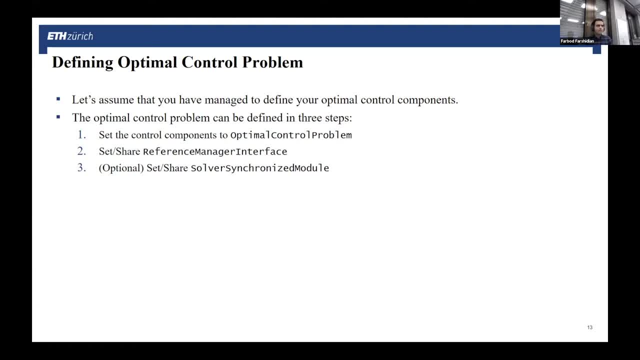 components to optimal control problem structure. then you need to define, set and share a reference manager and optionally you might define set and share some synchronization much. i will talk about these two components later, but let's start with the first one, which is, i think, more intuitive. but before that i like to say that we often take this three steps: 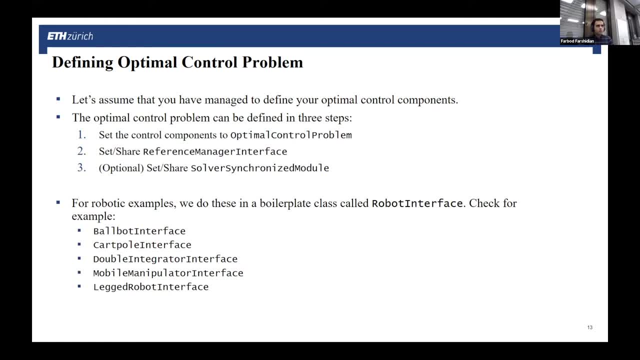 in something named robot interface. it's like a boilerplate code that we just implement our instantiate our optimal control problem and define the reference manager right. this makes it easier later on if you want to to again define your optimal control problem. you just instantiate that class. so for all the problems you have in ocs2 you will have one interface and 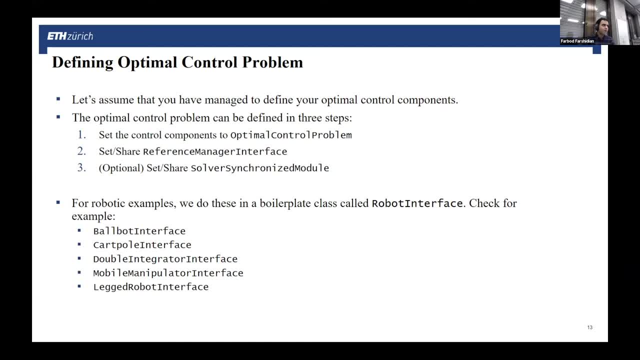 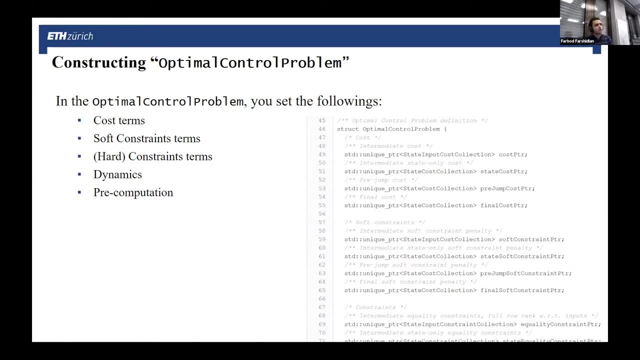 you can see these three steps are taken there. okay, now let's take a closer look. what is this optimal control problem? so optimal control problem consists of a couple of containers. so it has cost terms, soft constraint terms and hard constraint terms. then it has cost terms and pre-computation. so, one by one, the cost terms, as i said, you will have cost. 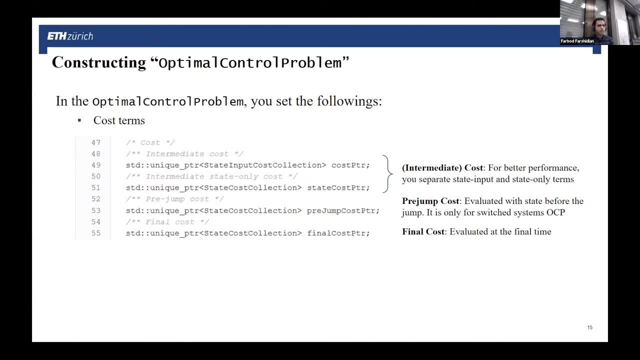 for three different time instances: intermediate, pre-jump and final one. as you see here, for intermediate we have two containers: one is cost ptr and one is state cost ptr. cost ptr is, in general, is a function of both state and input, while the cost state cost is just function of. 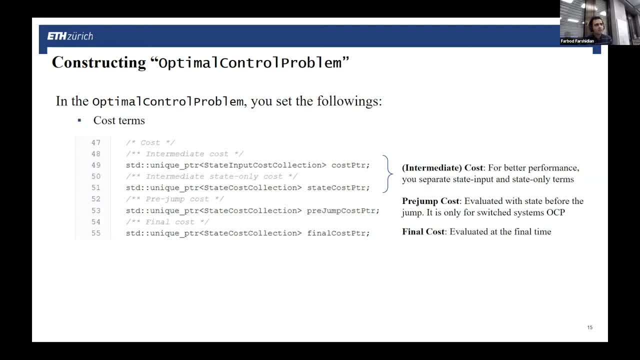 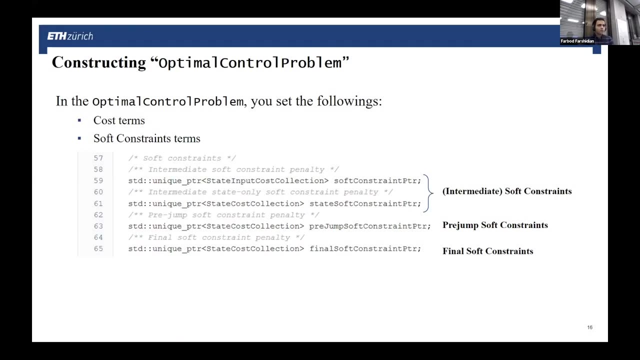 state. of course nothing goes bad if you implement a state only cost and set it to the cost one. just it's for efficiency reason that we separate it and you you can ignore it and just put all of them to the general. the second one is a soft constraint. i mean like if this, this is also if 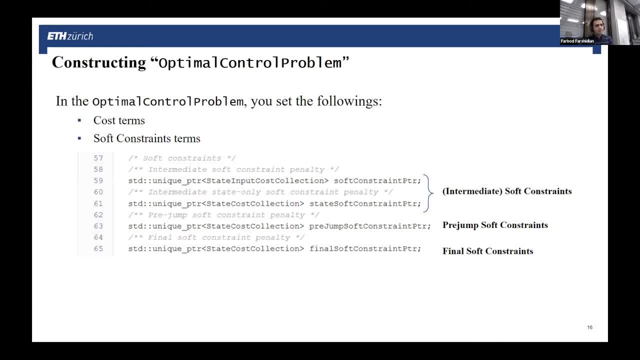 you have set of constraint that you don't want to handle them as a hard constraint, as a restricted constraint. you just want to have a softness, such as you have some collisions, you don't want to, you want to have some buffer and you just softly, just penalize them. so the soft constraints again. 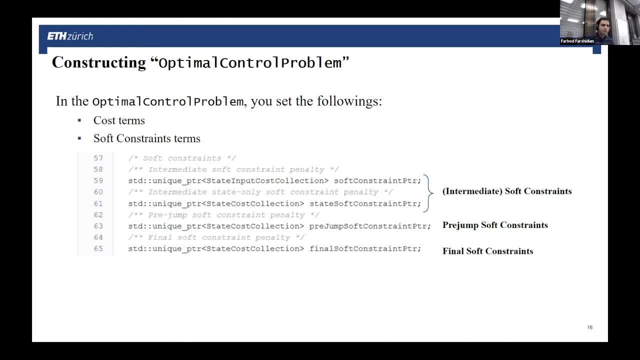 is for three time instances: intermediate, pre-jump and final. for an intermediate one again, we separated state only and state input soft constraint. now the question will should be asked here is how we should define a soft constraint. actually, ocs2 provides an helper classes which is 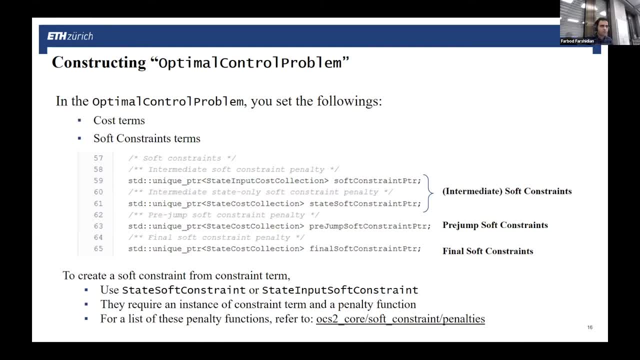 called state soft constraint or state input soft constraints. so in that that you create a constraint term, you define your penalty of your penalty function that you like, and you pass them to these classes and they generate for you a soft constraint term. so ocs2 comes with a list of different penalties but in general you can implement your. 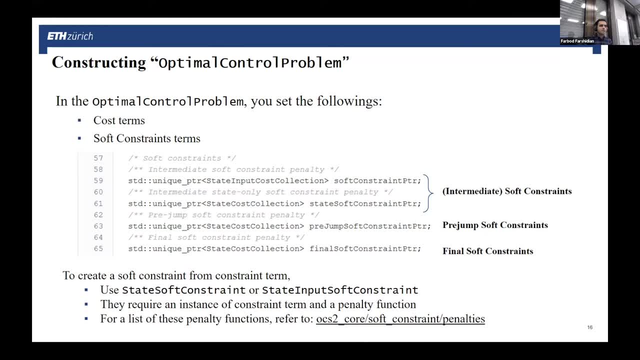 own penalty and use it. this, this, uh, this uh. separate, separating for each constraint, using different penalties. actually very useful, because you don't want policy, you want. you want to use different hyper parameters, maybe for constraint, or even different type of penalty for each constraint. so this gives the loss of flexibility for your design. now, after that, it moves to the 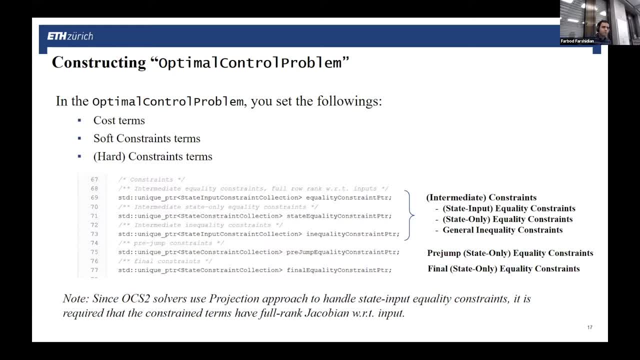 hard constraint. so for hard constraint again, three times three: intermediate, pre-jump and final. it's, it's, it's. we should notice that pre-jump and final are just state only, while intermediate one can be state or state, input or state only dependent, as, as i mentioned before, since we are handling state. 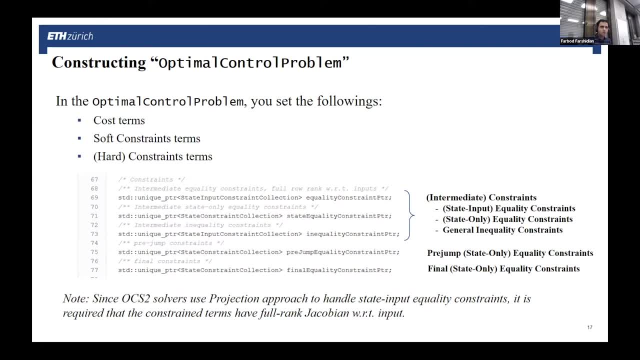 input equality constraints through the projection technique so you need to set them in a separate container. so you see that for the state input we have a separate container but for a state only quality and in general inequality- we have uh to other containers. you should notice, since we use projection, we you should guarantee that. 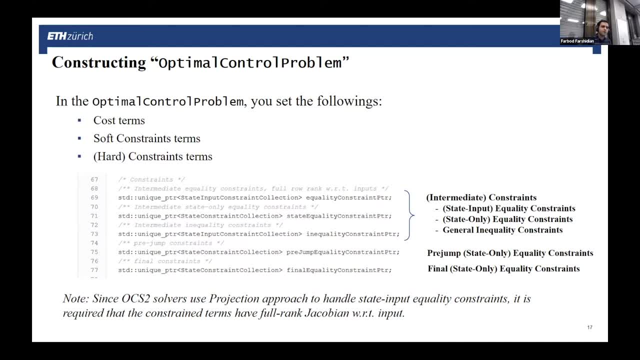 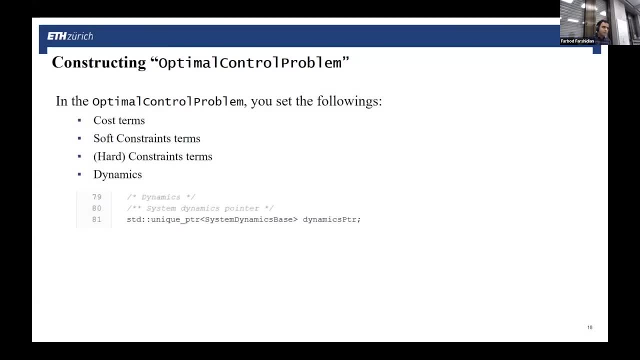 your state input, equality, constraint, stack are full row rank. if it's not the case, it's better you use the soft constraint technique. now this brings us to the simplest one, the dynamics. yeah, it's easy, just single field, you just set your dynamics and finally, something named pre-computation. 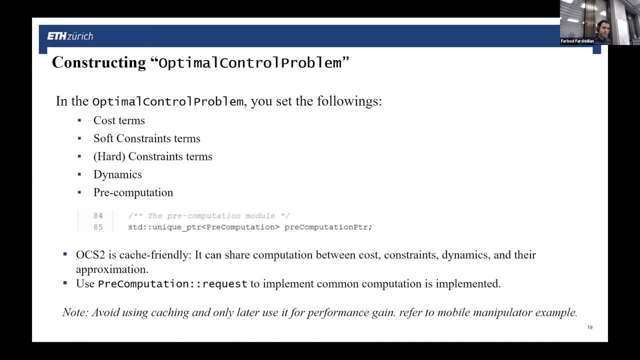 this is the part that i talked that ocs2 is cache free friendly. it means that it: this: this class allows you to do a computation that you can share between your cost constrained dynamics in that class. and how that works is solver sends a request message to this class and based on that request message, you decide what kind of common computation you. 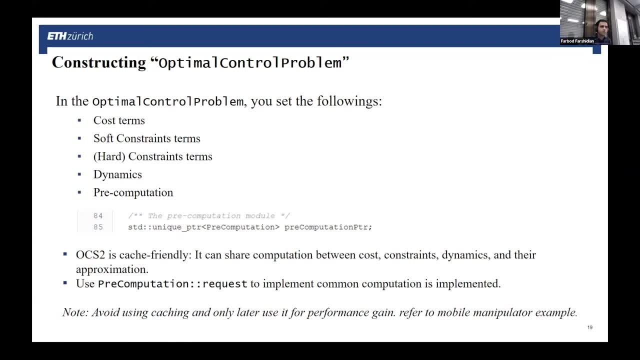 can perform and once that's done, this pre-computation instance will be shared between your cost constrained dynamics and you can use that cached value inside uh. so as a general rule, we don't suggest you to implement the cached version of the uh. your problem first. it's better you start with a non-cache version uh, because it's it's more. 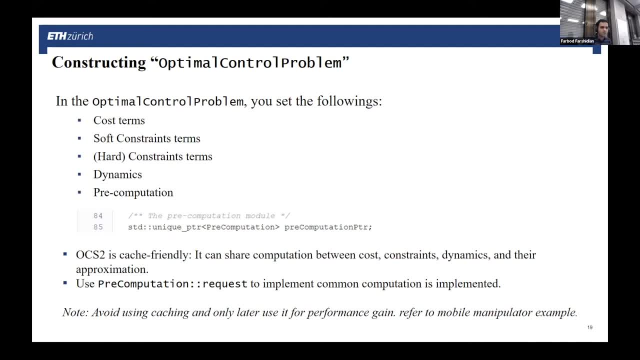 reliable. i mean it's less chance you make a mistake- often mistakes that you make. you will get it with the compiler but with the cache. once you have that for gaining more performance, you can use it as a benchmark and implement the cache version and make sure you get the same result. 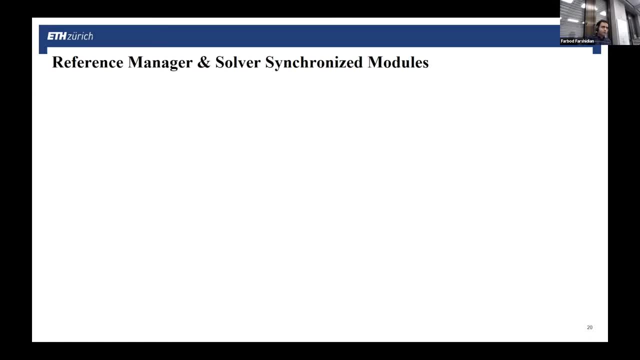 now, with this, we set up our optimal control problem we are. now we come to the two other steps that i said, that i'm going to explain it in more details- which is called the reference manager and solver synchronization modules. first of all, what are they and why they are needed? right, the reason behind it is more implementation from implementation point. 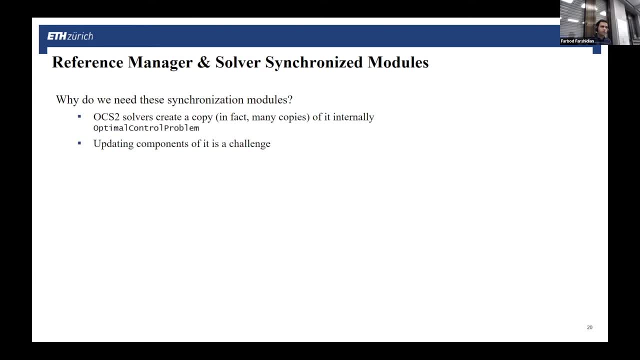 of view. so osu solver creates a copy of your optimal control problem. once you set your optimal control problem- the start that we just discussed- to that it creates a copy, actually many copies, of it multi-threading structure that he has internally. So if during your task you decided to update the 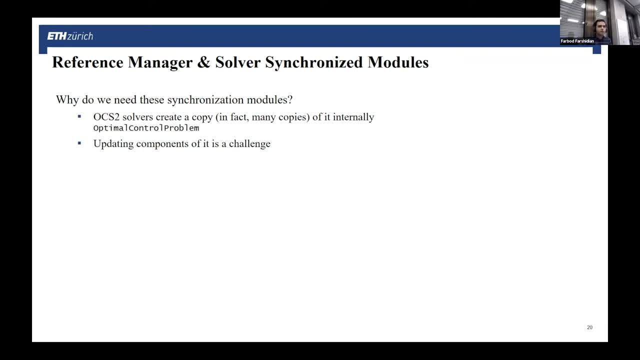 parameter in it. for example, imagine that you have a user-defined target and you want to update that. this would not be possible because you don't have access to those copies inside the solver. So to solve this issue, we introduced this concept of reference manager and solver synchronization. 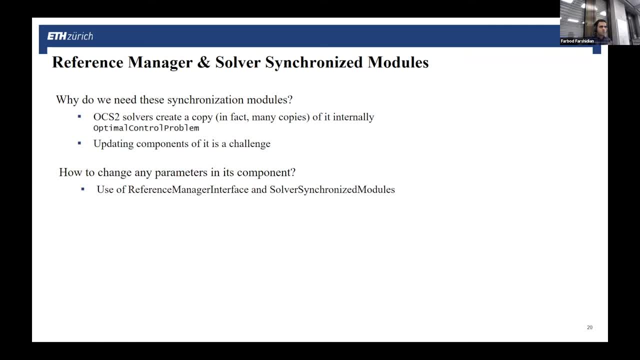 module, So the reference manager and the solver synchronization module. one of them is used for user references like the target trajectory you want to track and also the mode schedule that we discussed before, And the synchronization model is more general. for any other parameters I don't know: hyperparameter for your adaptive control or the map of the environment, if you. 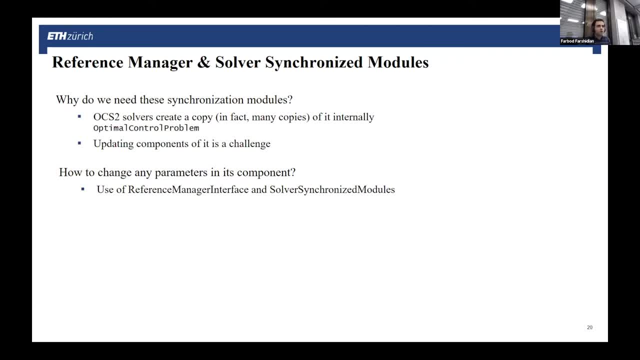 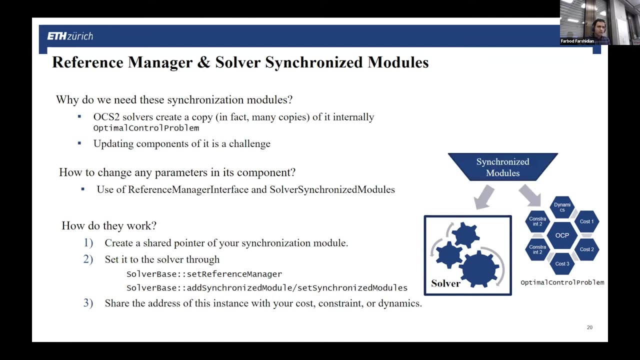 have a collision avoidance or you want to walk over a rough terrain. So let me explain how this works. So the idea behind these modules are shared memory. So what you do, you can create a shared memory of these synchronization modules and you set this both to your solver. 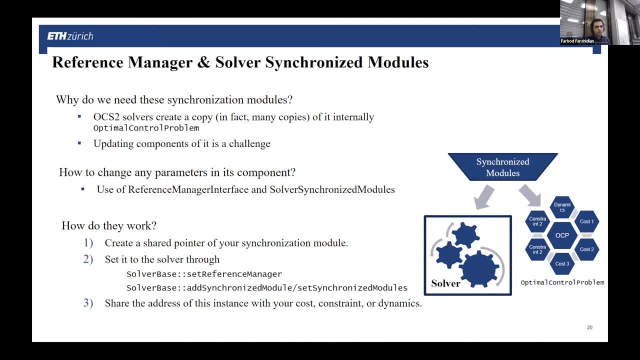 and to your optimal control component, Since there's a single version of this and this is shared between these. if now you decided to update the parameter inside these, you can easily just manipulate the parameter inside the synchronization module and it nicely updates all the other components. You should notice that you cannot definitely in. 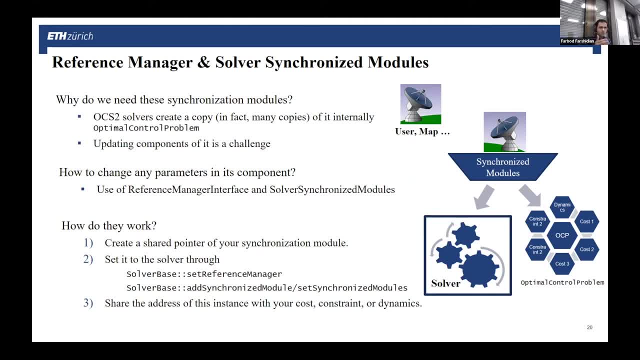 the middle of that change the parameter because, for example, you could be in the middle of one each other. So you can't change the parameter in the middle of all the other components. So you can't change the parameter in the middle of all the other components. So you can't change. 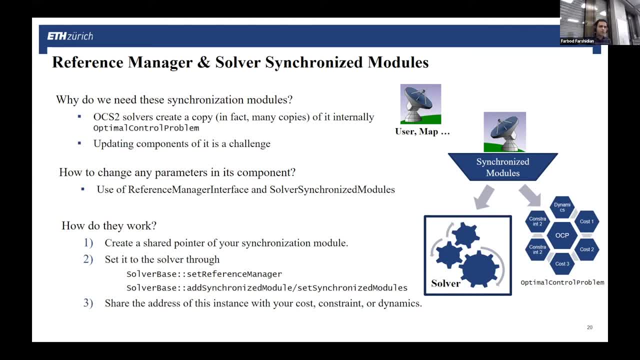 the parameter in the middle of all the other components, So you can't change. I don't know the mass of the robot and now the value is computed in one map and the other one calculated with the different mass. So to avoid that, actually synchronization modules take care. 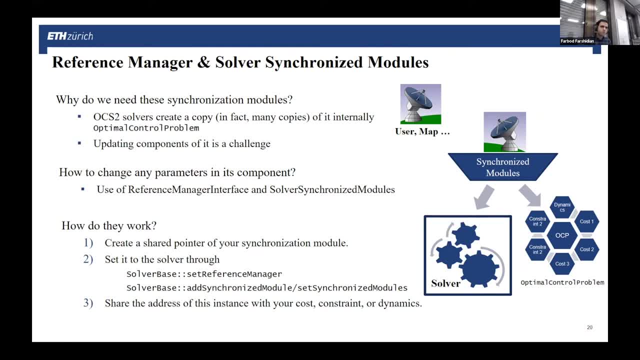 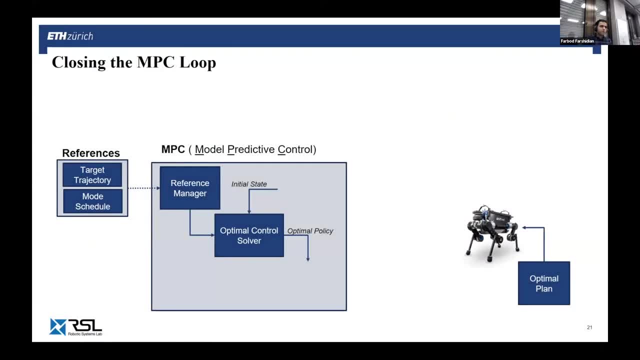 of the synchronization part for you. They make sure that they just update those parameters at the right time. Now, with having this you're done. You have your optimal control problem and all the modules that you need. So now you want to put this on hardware. 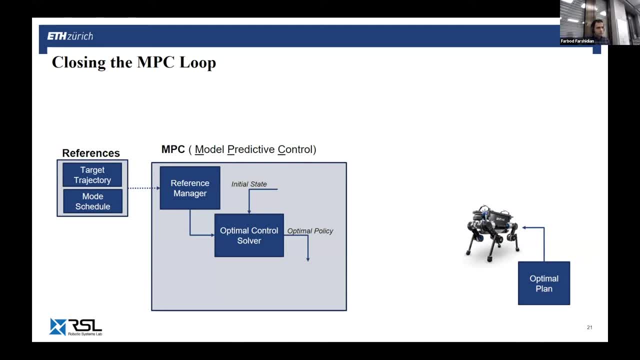 To do this, you have your optimal control solver, which you set your optimal control problem into it. You might have some ref, so you're going to get the initial state and it will optimize it and give you the optimal policy. You might have some references like target trajectory or what would 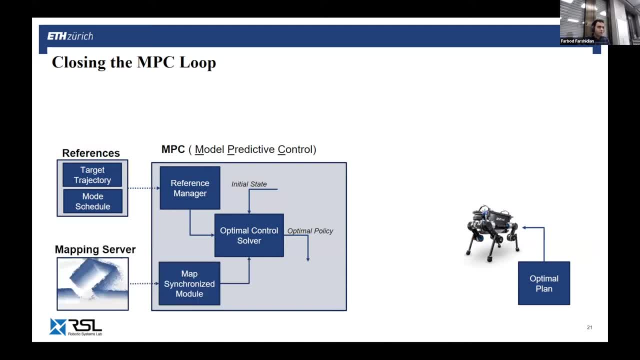 be the gate sequence or mode schedule of your problem. You might have some other solver synchronization model like map. Now the question is: how should I use this inside my tracking controller? Under this case, I'm going to use my tracking controller. I'm going to use my tracking. 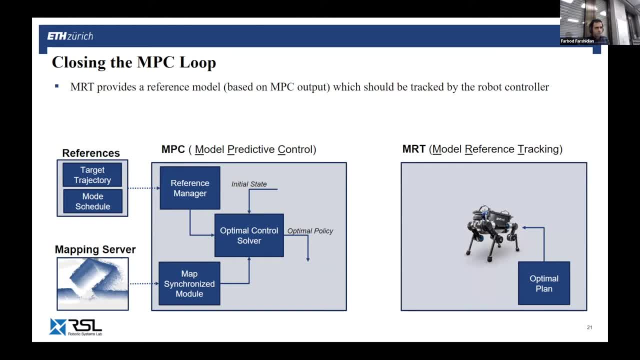 controller to track the state and input at the robot site. So for that we introduced this concept of MRT. MRT means the model reference tracking. It means that it's going to replay, generate the optimized references for state and input at the robot site. So what you need to do here, you need 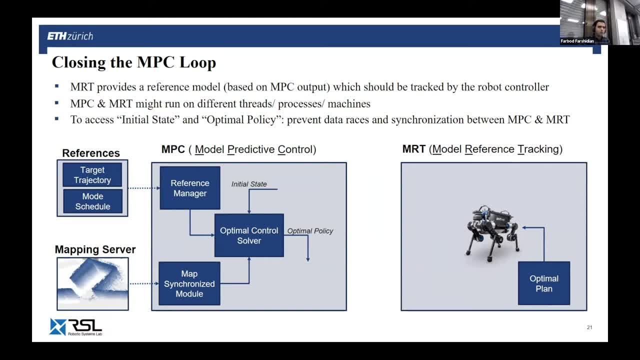 to make sure that this MPC and MRT are communicating properly together. It means that MRT always updates MPC with the latest state measurement and it reads safely from your optimal policy. This means that you should prevent data erasing because if you are suddenly reading the 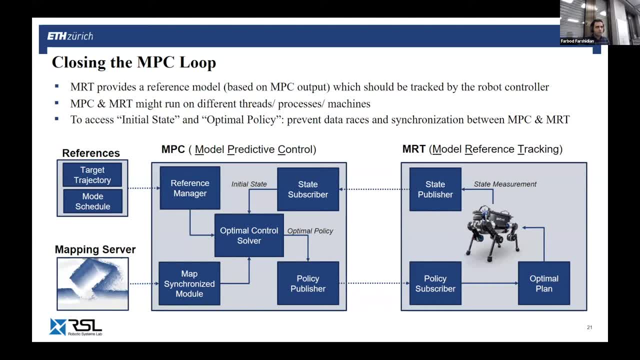 policy and MPC starts writing it because a new update arrived. this shouldn't happen And you need to make sure that you always, for example, use the latest state and you don't want to use old versions, As you see that here I'm borrowing terms from ROS, but this MPC and MRT has both. 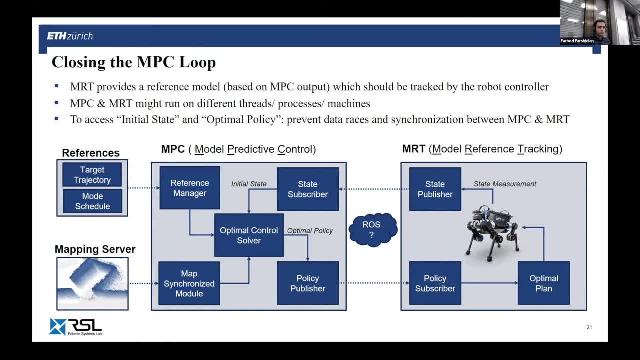 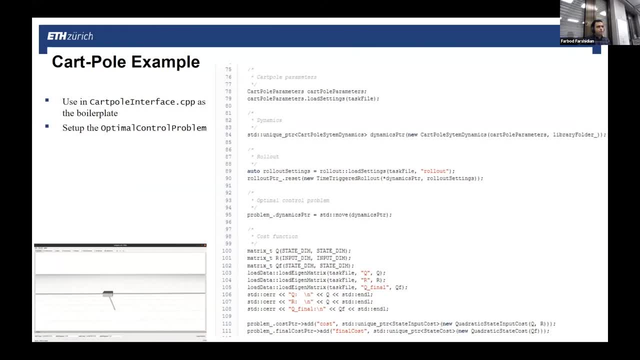 ROS and non-ROS versions. So for a non-ROS version, you can use ROS or you can avoid using ROS. That's a choice for you. Okay, now let's see a simple example here. So we will have the car, for example. It's a very famous control example, So you need to. 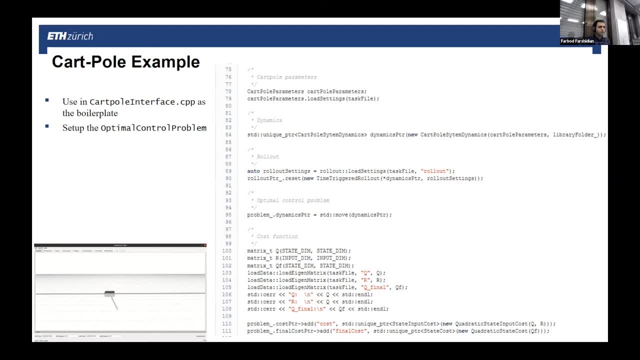 by accelerating, deactivating this car, swing up this pole and balance it there now. Now what you need to do with the first step set of your optimal control problem is: you define dynamics. here You see that we are defining the dynamics and the setting is the ultimate control problem. 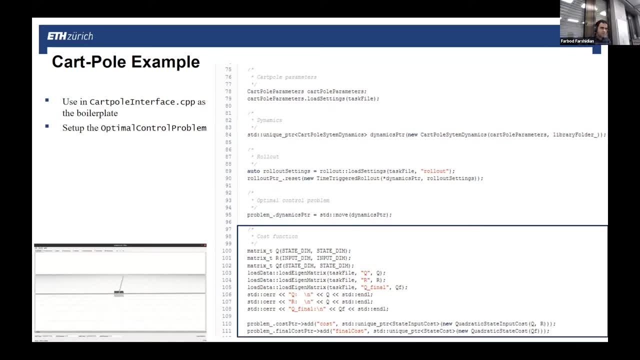 This problem is very simple. It has just a quadratic cost that analyzes deviation from the upright position. So you define a quadratic cost and set it to both intermediate and final cost. This problem doesn't have any reference manager or any more schedule, because it's a super simple problem. 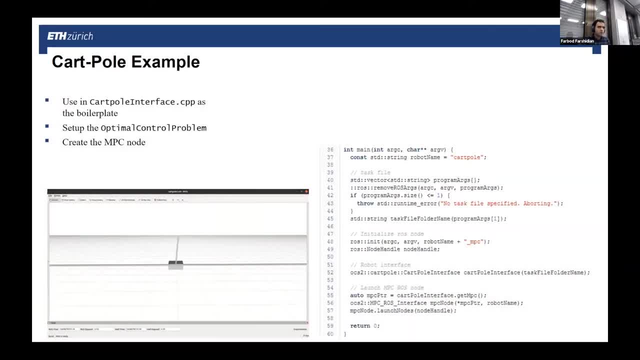 Once you did that, you have your MPC problem. So you can create the MPC and launch the node. Of course you need to write some visualization pieces there on MPC. The OCS also have some helper classes for that. but now you have your node. 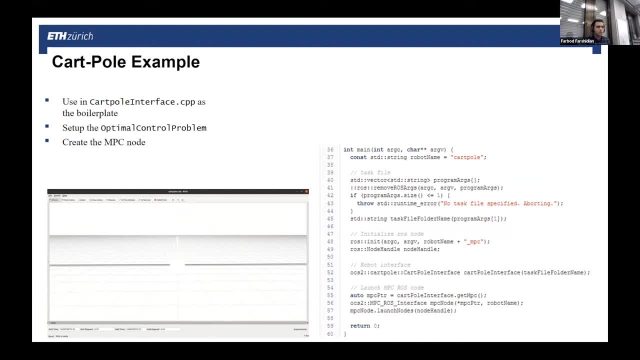 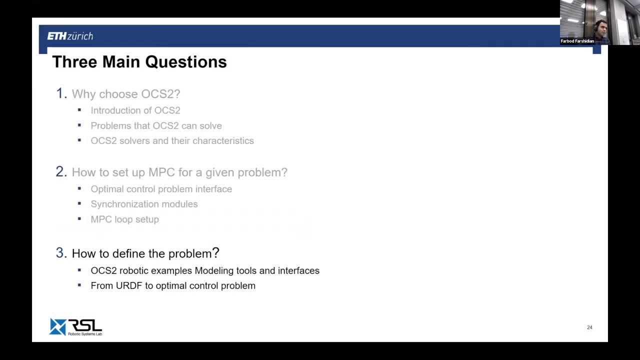 You just instantiate this and instantiate your MPC and you launch the node through this MPC-MRT interface that we discussed. Okay, this brings us to the last part of this talk, which is how to define the problem. Now. so far, we assume that you somehow have. 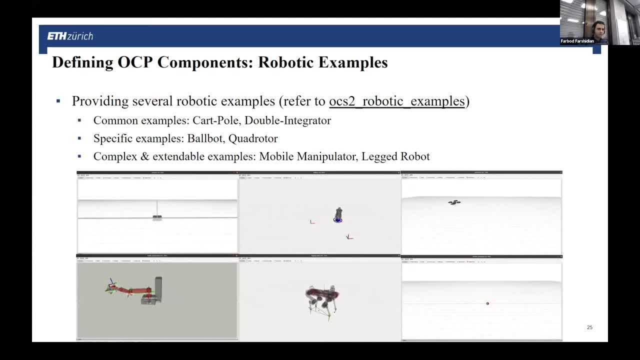 that optimal control problem components: right. You have somehow drive your dynamics, somehow drive your cost, somehow drive your constraint. Now, in reality, I mean, you need to do it somehow right. One way to do it is through cheating, right. 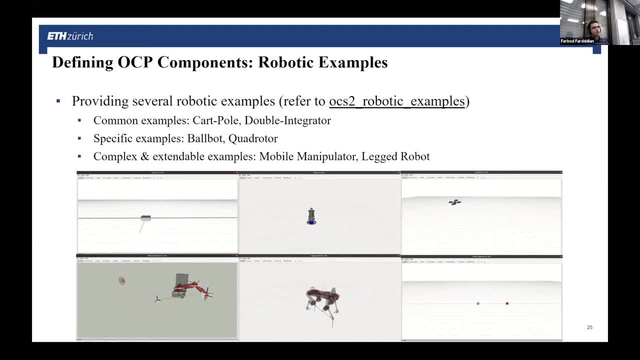 Let's say OCS2 has six different platforms in it which you can look into that and see that, which features you want and how they are implemented, and just get inspiration from them and implement in your code. The documentation page gives the details of specification. 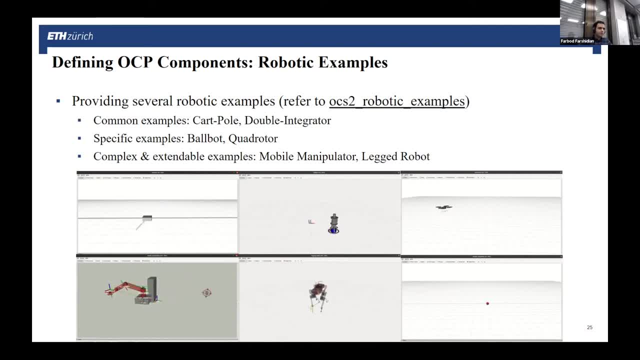 of this, of this example. I mean they're covering from the legacy system to a mobile manipulator, with the self collision avoidance, and also some toy problems like this double integrate. But maybe we can not cover everything right, So there would be something. 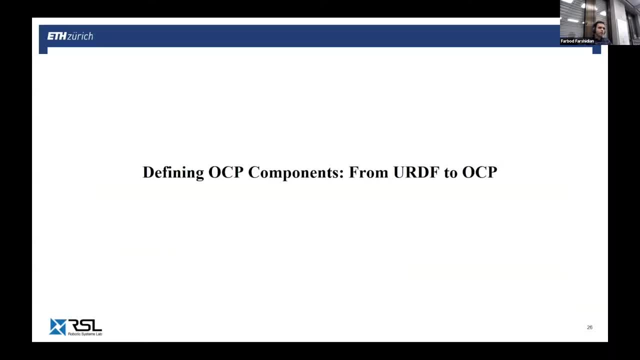 that would be specific to your robot. Now the question is how we can help you to actually define those. So here is the, the idea. we want to provide some sort of helper classes to you. that from your general description of the your, your robot, let's say that your idea defines specific optimal control components like 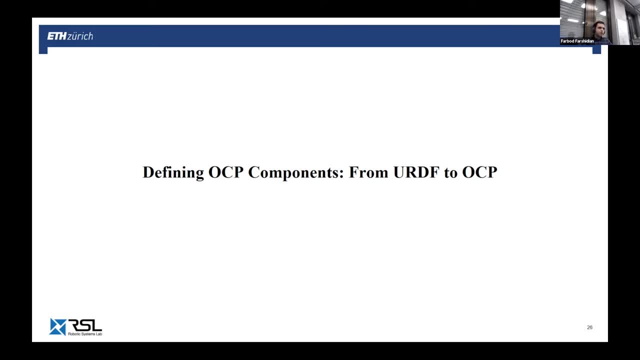 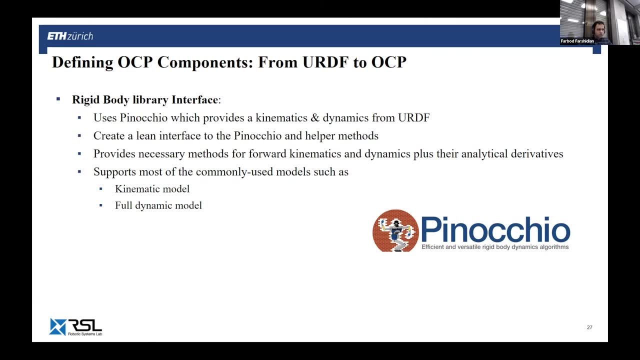 your dynamics or your constraint. so for that, uh we are. we. we have five different uh uh tools here. first, we need to create a nice interface, an interface to a rigid body library that is capable of doing that. for that we are also using Pinocchio. so we are, we are creating a linear interface to 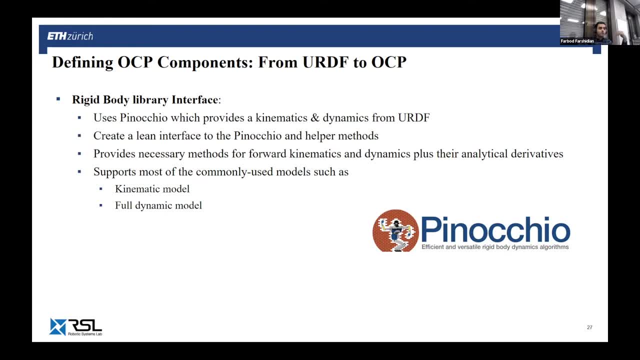 the Pinocchio uh which, with the nice thing about it, with the URDF model you can get your kinematics and dynamics and this means that you get support for very most of the commonly used uh models. like, if you have a full dynamical model or a kinematic model you can easily, by Pinocchio, generate. 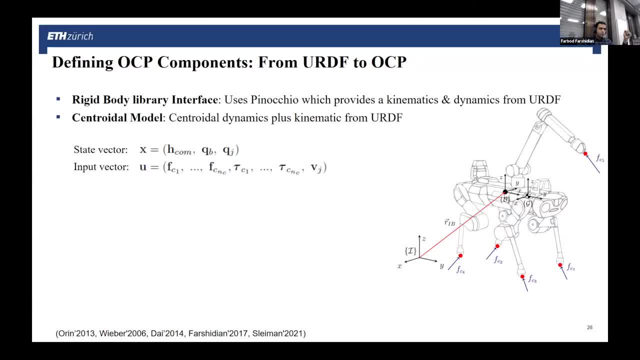 uh, we also provide some support for a bit more unconventional models like that, the Centroidal model. if you participate- if you have participated over talks from Scott or Marco, you have seen this. this sort of model, Centroidal model, is used extensively for a Lega system robot. the idea: 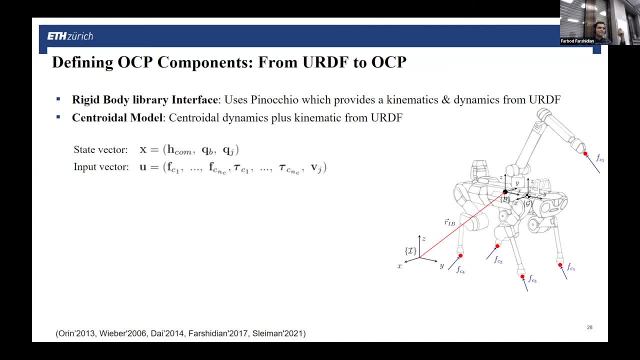 behind this is: you have a model which just contains the Centroidal dynamics plus the kinematics. so what we provide here for you is a class, a helper class, that gets the URDF and the name of of the contact frames and generates for due to dynamics. 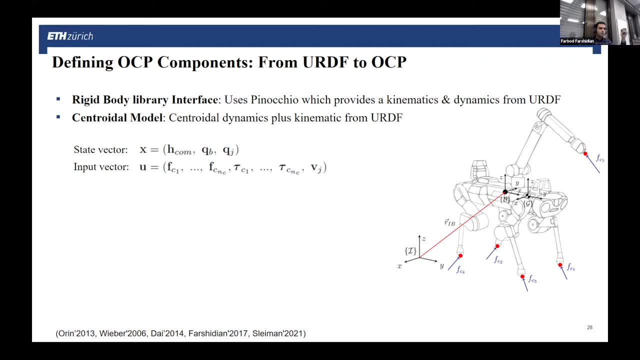 So I go very briefly what this model look like. I mean the states are the angular and linear momenta plus the pose of the base, plus joint angles, And it's action space or input vector is the 3D and six 3D forces and torque, and at the contact points, 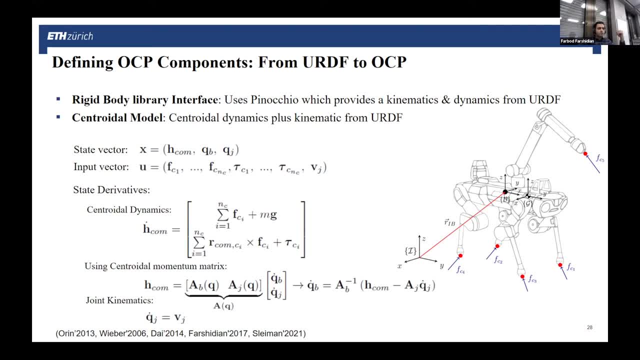 and velocity of the joints. So the derivatives are defined based on centroidal dynamics, which is the Newton-Uehler technique. The centroidal momentum metrics is used to define the derivative of the time, derivative of the pose, which you see, that is also incorporated. changes in the changes coming from the velocity of the limbs. 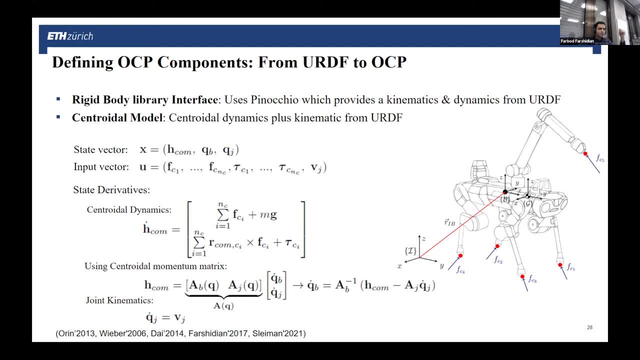 And the final one, joint kinematics, is a very simple map. So all of these stuff are. we are using Pinocchio to extract the centroidal model and the the centroidal momentum mapping, And we created some helper class for you by that. 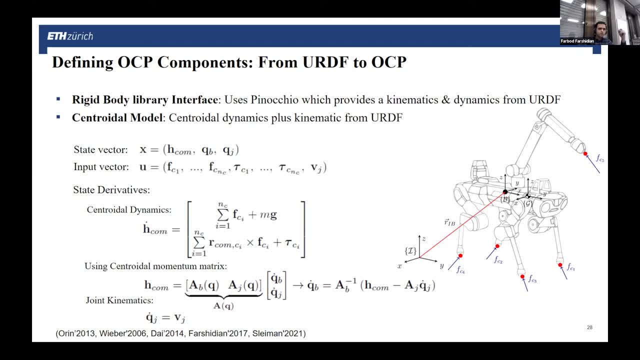 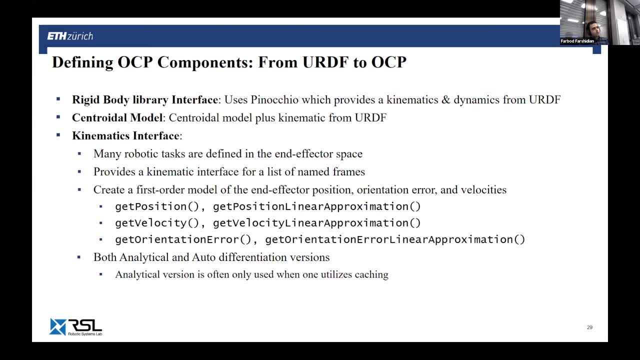 with a single URDF you can get this full model for your legacy system. Now the third tool that we provide is kinematic interface. So in many robotic tasks you often have the problem that you want. you'll have a problem that you want to define. 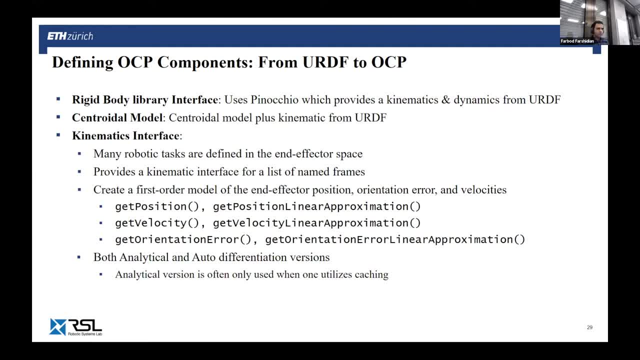 some end. effector space costs like tracking or integrated constraint that your stance stands for shouldn't move on the ground, So that means that you need some source of model to then the factor that gives you, for example, its position or its velocity is this, or its orientation and also its approximation. 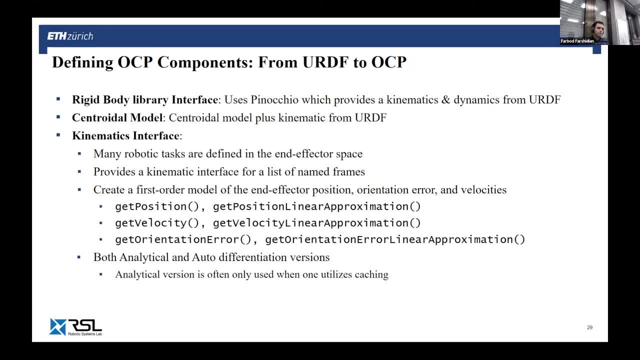 because for defining cost and constraint you need them. So we do this with our kinematic interface and we provide both analytical and auto differentiation version. And finally- I mean my finally- comes to this self collision avoidance. This is one of the missing part in many robotic tasks. 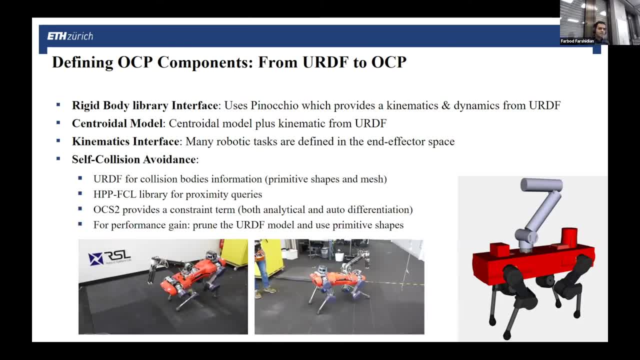 This is one of the missing part in many robotic tasks. This is one of the missing part in many robotic tasks- robotic tasks that are using MPC- because often defining such a constraint are very difficult and it's not straightforward. So, since we have seen this problem, it happens in many different- 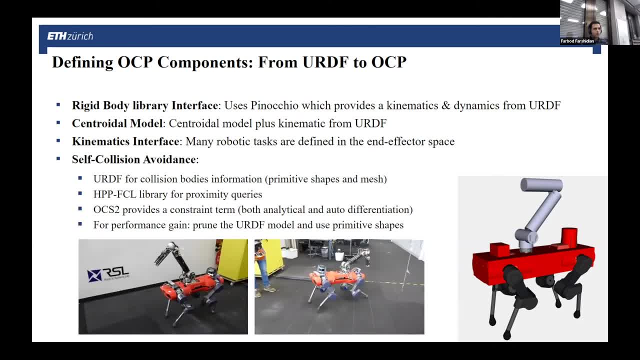 tasks. So we decided to create also a general interface, that from a URDF model. it gives you a set of constraints for self-collision avoidance. How it works: it uses the URDF and its collision body information, primitive shape and meshes, and it uses HPPF, CLN, Pinocchio library for 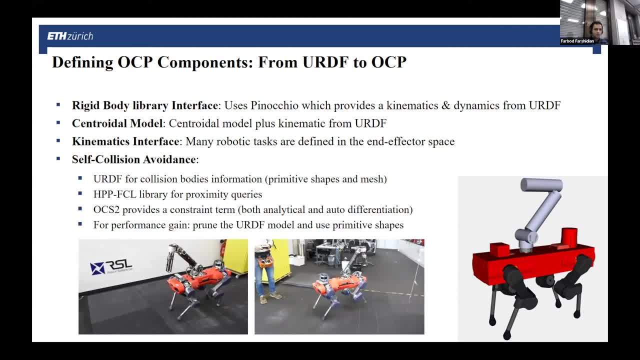 proximity queries and calculating the Jacobian of this distance- shortest distance to the nearest collision body- And then OCS2 automatically defines for you a constraint term. So therefore, from the URDF you get this self-collision avoidance constraint terms that you can set. 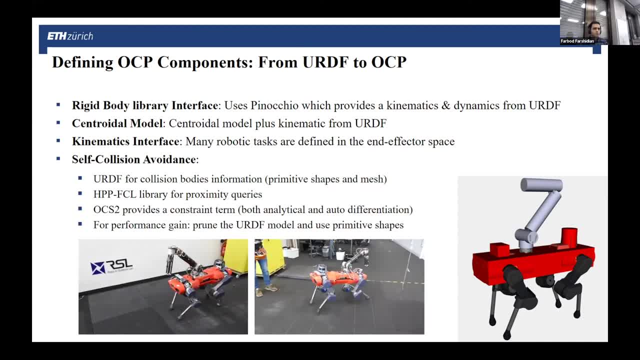 to your optimal control problem. Of course, for performance gain you might want to prune your URDF, For example with this animal C robot for a base. we had many collision bodies for just the base, the torso of the robot. But in the end, what we did? we just simplified it with a box and two boxes and one. 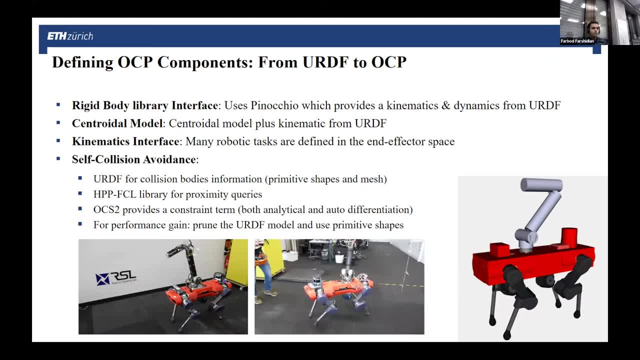 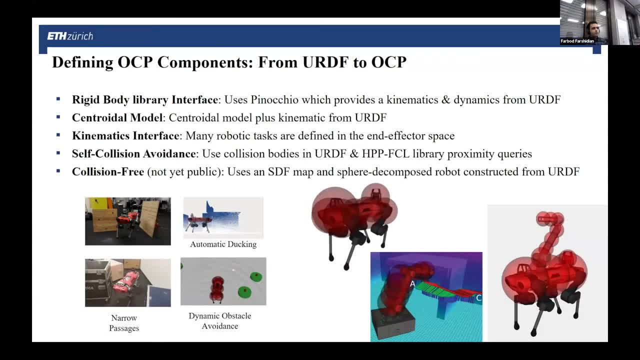 cylinder, which helps a lot for calculation of this distance. Okay, Now the final component is a collision-free. This property is not yet public, but it will get public soon. Then I mean, after self-collision avoidance, we want to also make sure that. 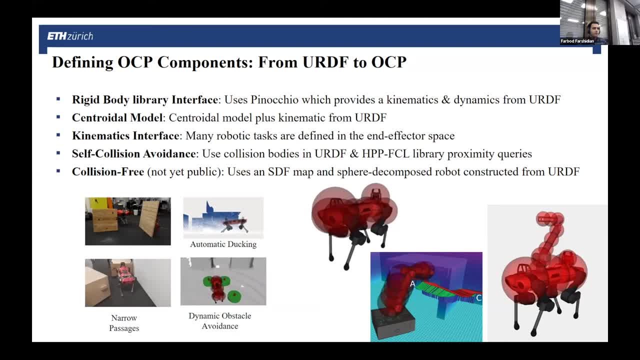 your robot does not collide with the environment. So for that we are using an SDF map server that generates you the science distance field And automatically from your URDF file we decompose the robot into this. This is the URDF. This is the URDF. This is the URDF. 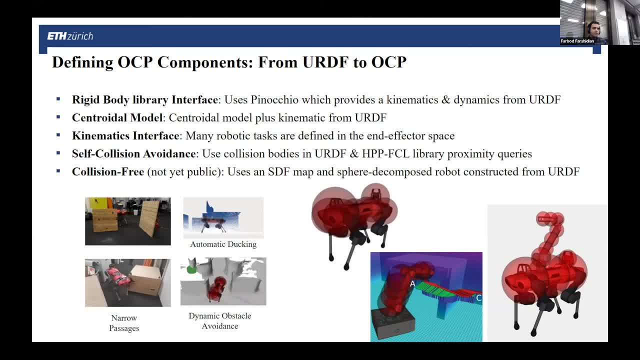 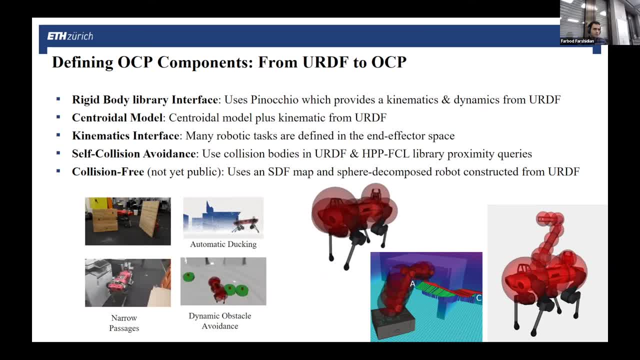 take care that our DC springs are typically Compact, and that's a lot to take care. We beefed up these primaries now because we have this M saturated matrix that could work well with a system that would work very well, in fact larger than also a system with these. 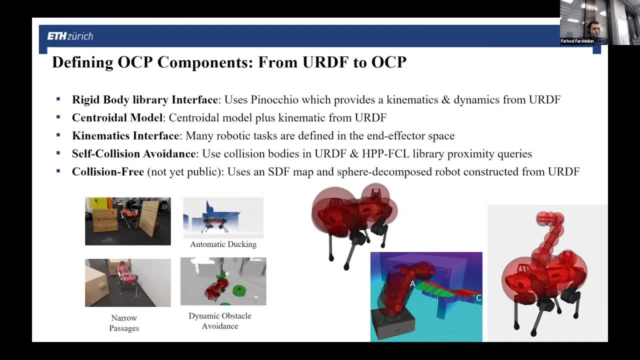 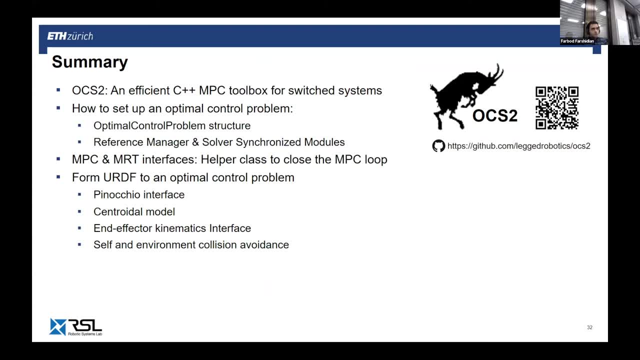 large orders. idea was coming from URTF, the OCP. So, in summary, we talked about this OCS2 as an Efficiency++ MPC toolbox for switch systems. We talked about how to set up the optimal control problem by defining the optimal control problem. 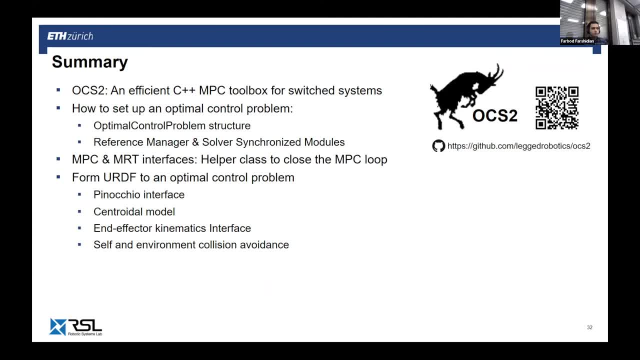 structure and this reference management solver synchronized module. We also showed that how you can use this MPC-MRT interfaces as a hyper-classes to close MPC loop on your real hardware or in simulation. And also we talked about this concept from URTF to get optimal control component using 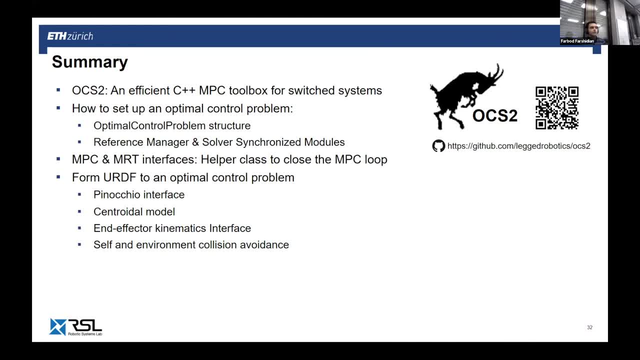 Pinocchio interface and fluid dynamic model and end-effect telematics and self and environment collision. With that I'd like to close. before closing my talk, I'd like to thank our developers team. So from left to right is Ruben. 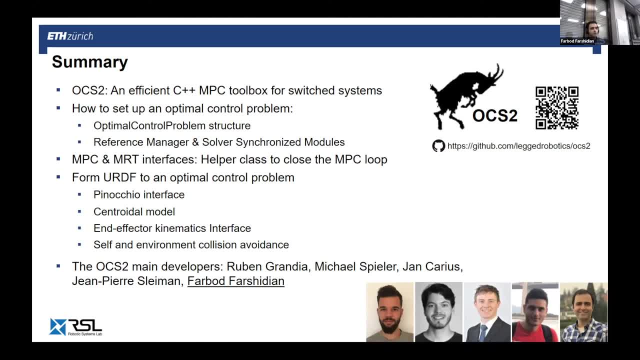 Garandia- he is a PhD student in our group- and Michael Illich-Piller, a former software engineer of our group. Jan Karius, former PhD student and newest member, Jean-Pierre Soleiman. And the last one is me, and which I'm also part of. 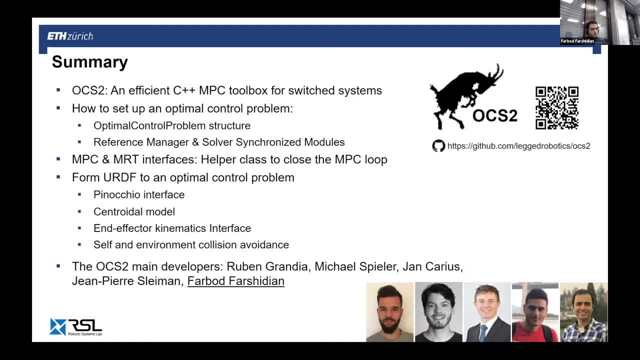 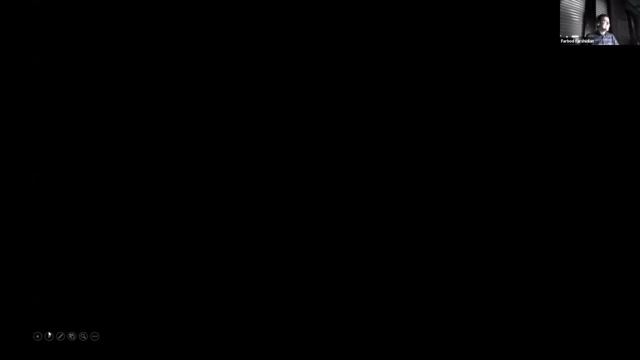 the developer team and also the manager of this project. With that, I'd like to thank you a lot for your kind attention and I will be happy to take any questions. Thank you very much for your time and I'll see you in the 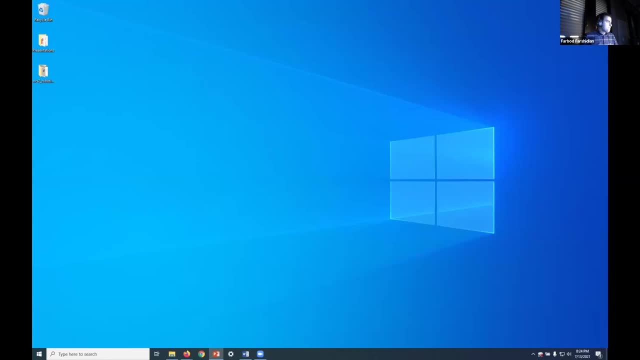 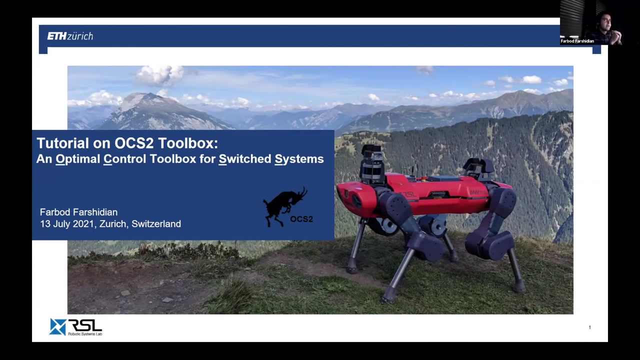 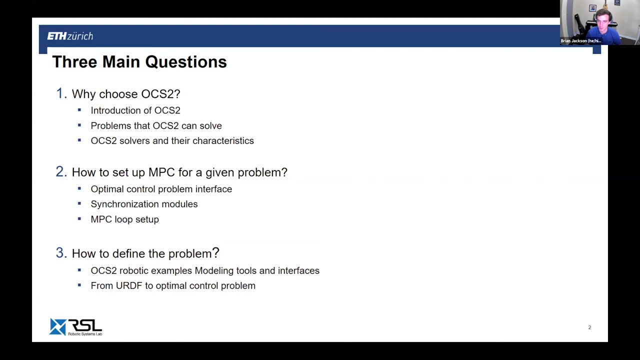 next session. Do you want to get your questions into the chat? I have a question for you, Farbaud. What all are you parallelizing Like what? yeah? what pieces of the problem are you competing in parallel and what's still kind of inherently? 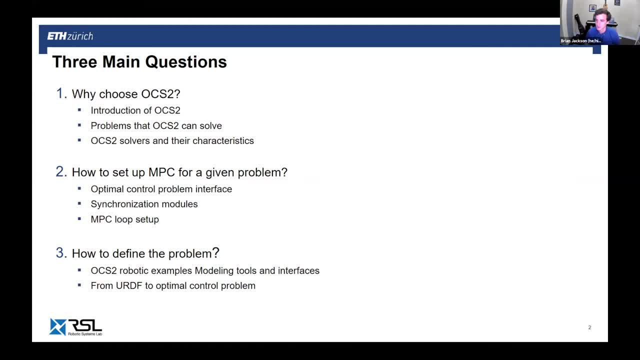 serial and what are, like, the current bottlenecks in your computational approach? yeah, so the, the linear quadratic approximation of the problem is the linearizing dynamics and constraints are happening, or in parallel, uh, the, depending on the solver, this, the answer changes. so for tdp based methods we also use, uh, we are defining some, some we are breaking down our horizon into. 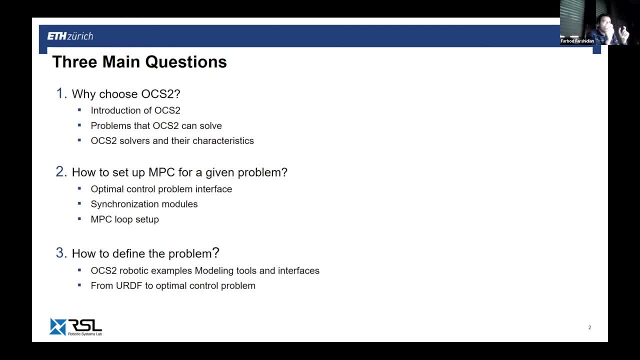 smaller uh pieces and we solve the ddv problem each of them and make and make sure that we have this connectivity. uh constraints for the ddp, for multiple shooting, sqp, this, this doesn't happen, but this everything happens in one run. and yeah, and search strategy are often 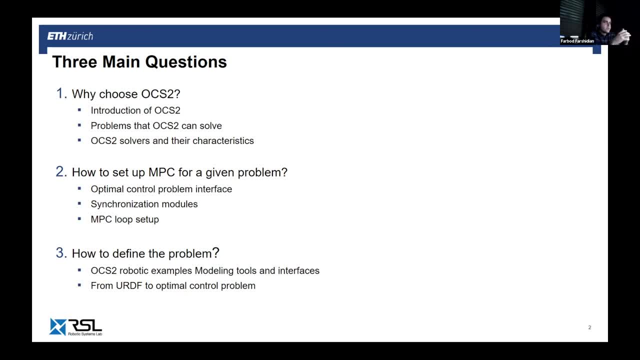 happens in the, in the parallel, because you need to search over different step lengths, um, so that's why i wanted to do that, and then i guess i'll be back and we'll go into that, but we'll get to that later. um, so this is uh, this is a. this is a really interesting thing to do. 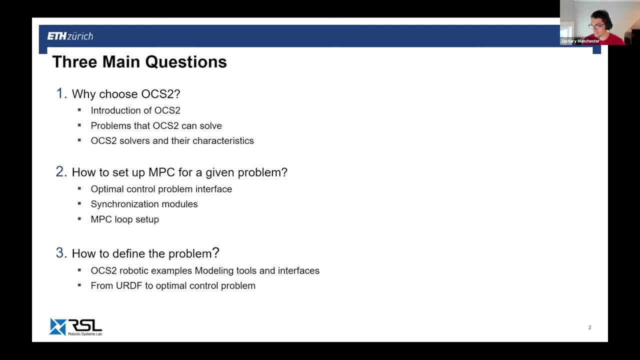 i have a question about the frequency dependent stuff which i checked out a while ago and this was it's. it's a cool idea and it's something that, um, that i feel like is sort of there as a heuristic all the time in a lot of things we do. i'm wondering, like, uh, formalizing this a little. 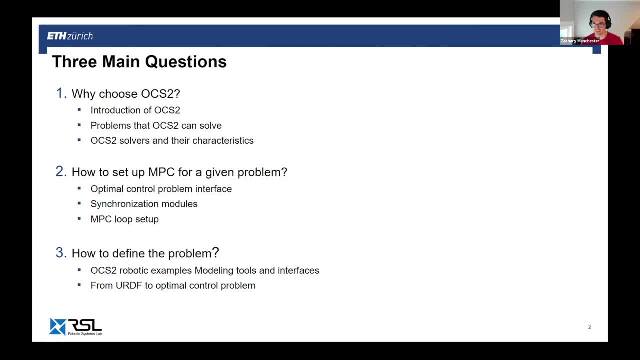 bit more is something i've been really interested in. do you see like an interplay between this and like um the lower level control- and i think this was something that came up in the last talk as well. this idea of like how does MPC sort of interact with the lower level controller, I think is a very 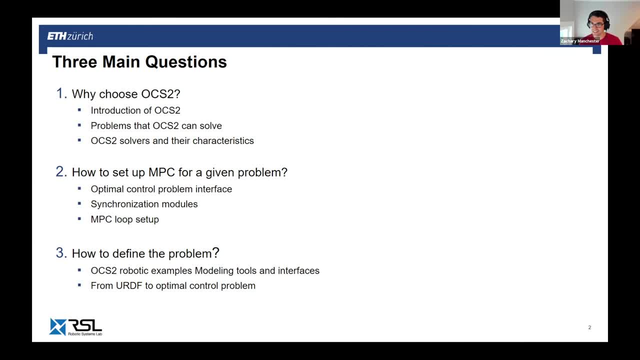 deep question that hasn't been really well studied in our community and like this is yet another sort of like you know thing in that direction of like needing to reason about the lower level controller, um, in the MPC, you know, in this case, and in sort of the smoothing uh, but uh, yeah, I guess, thoughts 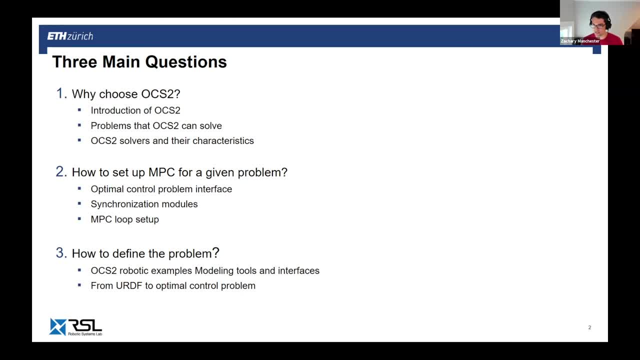 on this in general, like, um, this lets you use, I guess, the LQR gains more effectively, but, uh, I think the same sort of thing would apply with any lower level controller, right, yeah, that's true. so this, this, I mean, uh, this allows us also to, because we did this study, we showed that if you, if you. 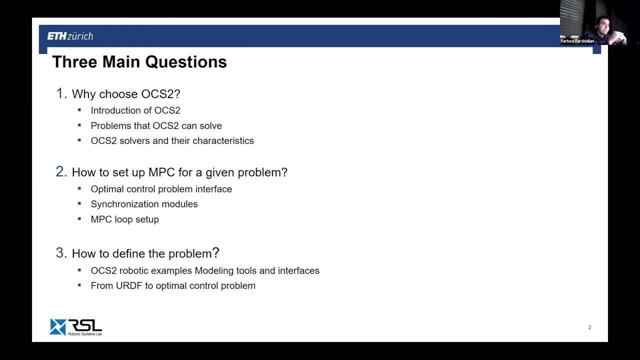 this approach, you can actually significantly reduce the amplitude of the feedback, and it comes from LQR, and then you can actually use that to feedback your, your, your, MPC, between two updates. right, you can. so now we can easily go lower to 30 hertz, as you said that this is one. I mean, uh, this. 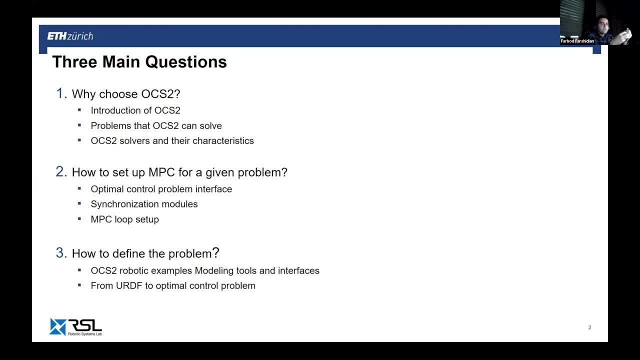 is one outcome, outcome of it. so we just uh smooth in this LQR gains but in general, also the feed forward solution, the optimal state and input trajectory getting very smooth. uh yeah, I think that the main reason behind introducing is low level tracking controller. right, this, you cannot track anything. 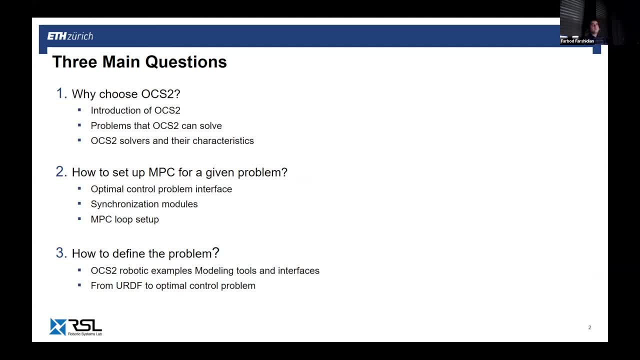 that we generate, and this comes from our understanding of how well our low level controller works. we often just, uh, we look at the bandwidth of our controller and try to tune them more or less based on that values. but to say that sometimes it goes also the other way. you can. 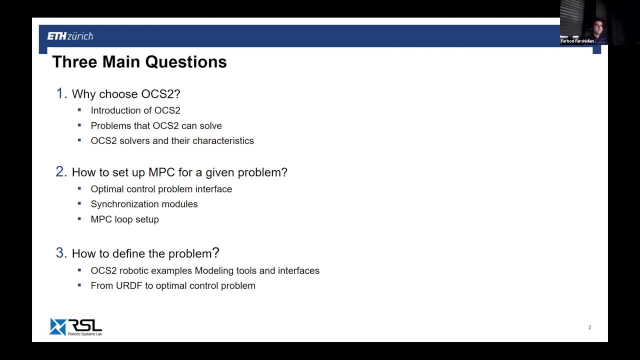 sometimes encourage to have a high frequency uh content in our solution, for example, you have a loss of restriction friction and you want to break them and otherwise if tracking controller will not work well, and then you actually do the reverse. so you're encouraging for high frequency solutions. 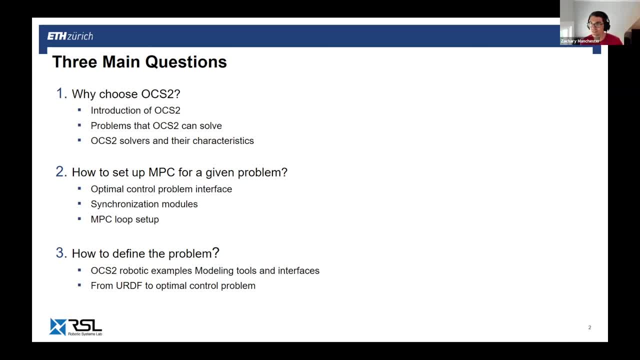 yeah, thanks, uh, anybody else in the audience? yeah, Ibrahim, hi, do you hear me? yeah, okay, uh, thank you for the nice presentation. I have a question about the initialization of the software in general, like I'm a user of the of OCS2. 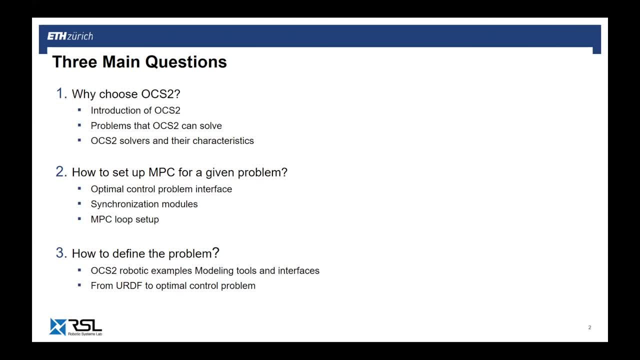 and I don't quite fully understand how the MPC solver is initialized. Yep. so this is an interesting area, right? So, in general, OCS2 requires you to define your initialization yourself, So you have something like initializer class which most of the solver require. 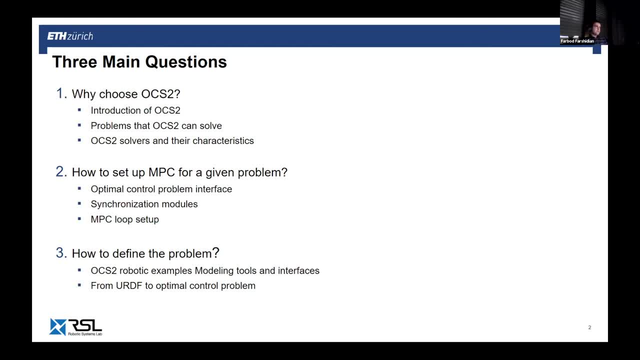 which will give you starting and final time, and you need to somehow come up with initial solution For many of this task and the implementation that we have. we are simply using the current position of the robot and we are assuming, over the time horizon, that it's keep the same thing. 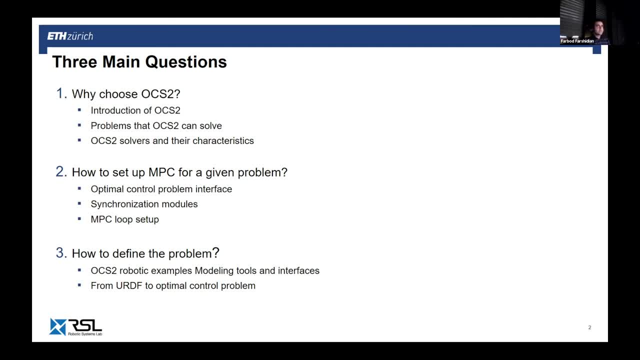 But if you have, for example, a legacy system, you also make sure that the contact forces are good for static balancing. It often is enough, but you can imagine that can have a significant effect on the overall performance of the robot And finding a good local solution right. 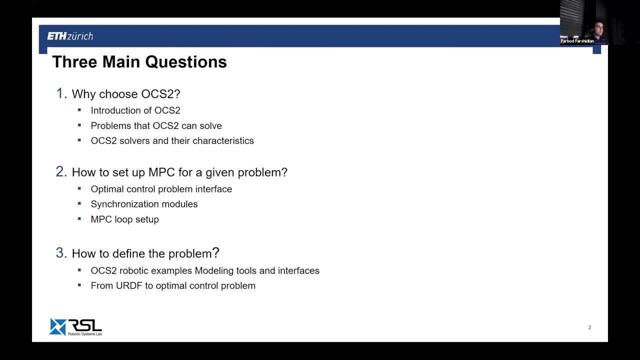 Because with a good initialization you can skip that local solution and go to the next one. This can be addressed through some sampling-based method or some reinforcement learning technique. that just propose you an initial solution And from that point MPC starts to optimizing for more optimal and feasible solution. 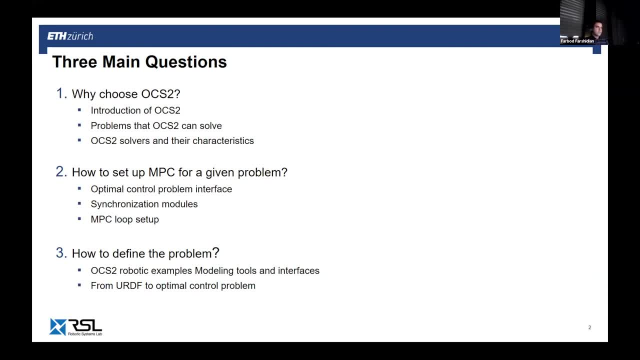 So, again, OCS2 leaves this to the user, So it has this default behavior. If you don't want to define your initializer otherwise, you need to implement this as well. Okay, thank you, All right. So thanks a lot, Farhud. 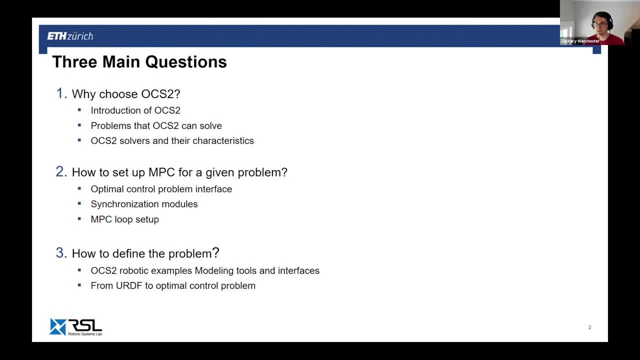 That was great, And I guess it's just about time to switch over to the last of the tutorial talks. So